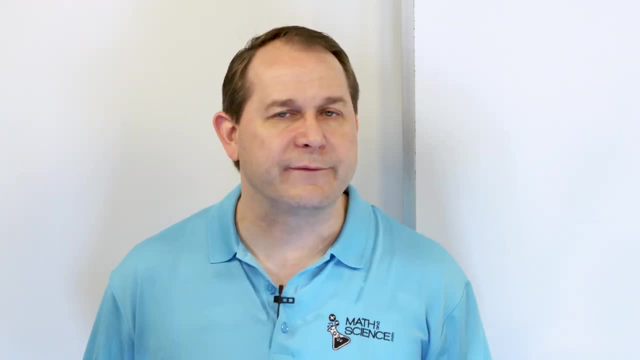 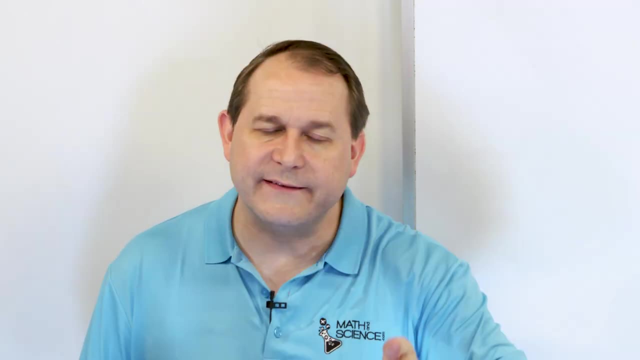 where to put the decimal point. So really it's not going to be any different or very much different from what you already know. Second thing is, when we were adding and subtracting decimals, I told you you must line up the decimal points. I told you, 30,000 times when you add or subtract to line 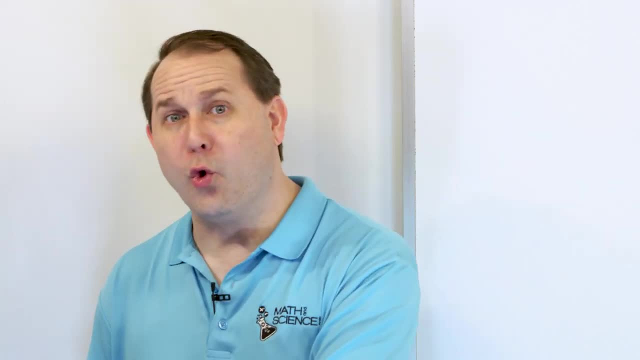 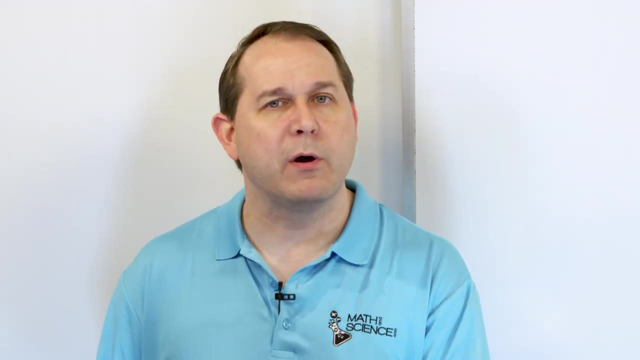 the decimal points up When we multiply or when we divide. we do not line up decimal points. The lining up of the decimals only is for adding and subtracting. Here, when we multiply, we do not line up decimal points. We don't do that. So let me show you how we're going to do. our first, 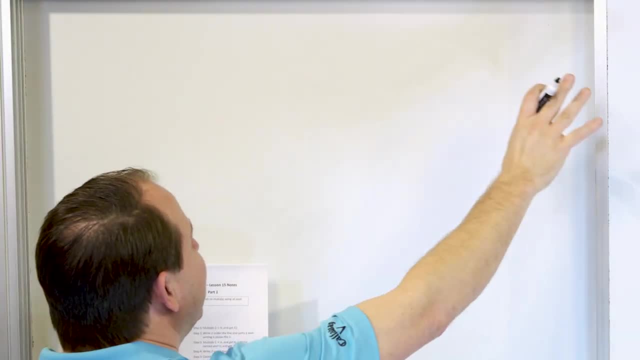 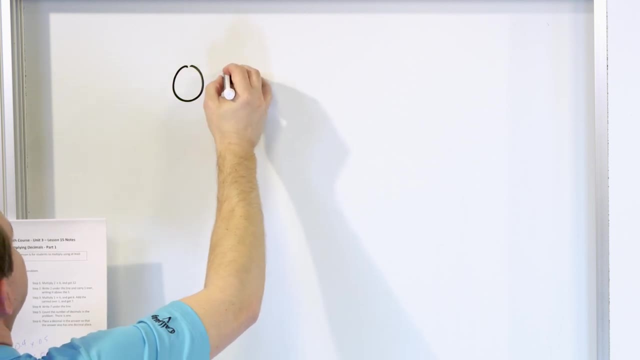 problem. This problem actually is the same problem we did in the first lesson when we did by the models. here We did a problem that looked like this: 0.4, and we were multiplying by 0.5.. 0.5.. Now in this case the decimal points happen to line up, but I'm not lining them up on purpose. 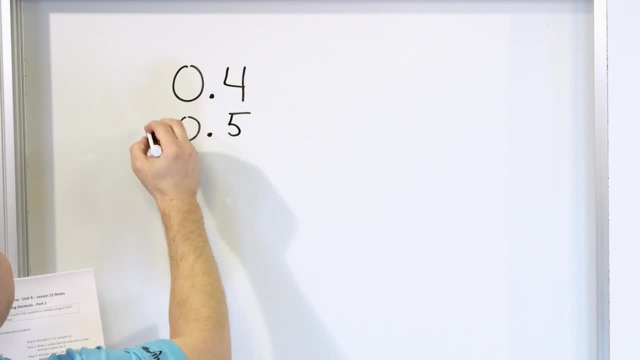 I'm just doing it because the columns are lining up and the decimals happen to fall. here We're going to multiply. Now, if you remember from the last lesson, we said that basically you just ignore the decimal point until the final answer. So what I want you to do is just pretend the decimal isn't even there. 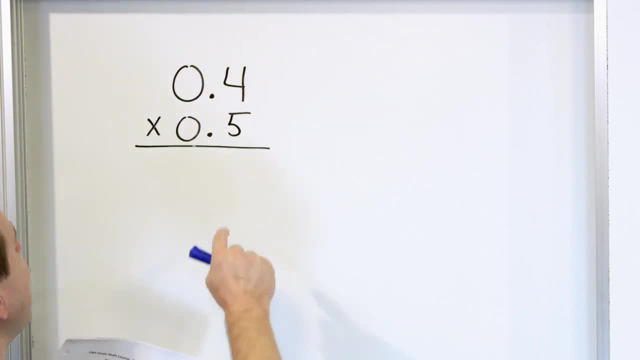 Like, just pretend it's 0.4 and 0.5 and we multiply. What do we do? We start in the right column: 5 times 4 is what? 20, right? So we put a 0 here and we carry a 2 over here. Then 0 times 5 is 0, and then 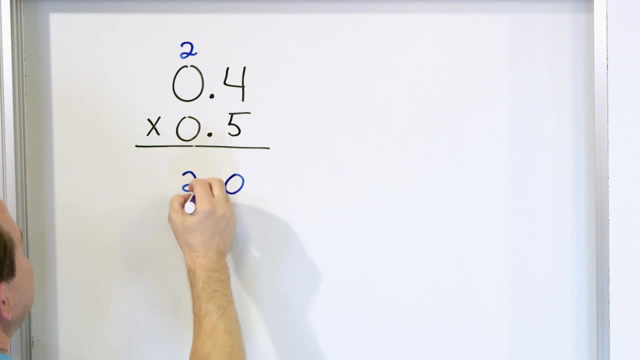 we add the 2, which means we get a 2. So we put a 2 here. All right, now we're done with that. So then we have to multiply by 0. So we can drop a 0 down here, and then we multiply 0 times 4 and we 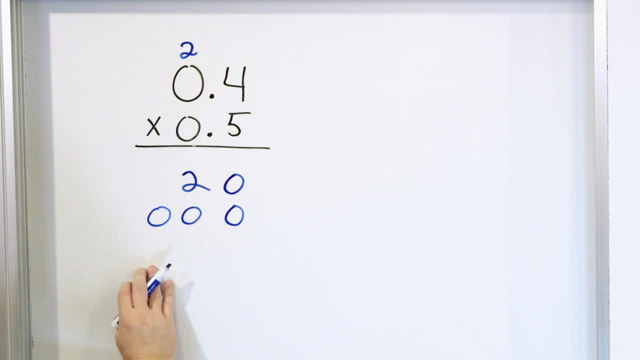 get 0.. And we multiply 0 times 0 and we get 0.. We don't add this 2 because that was from a previous step. Now, whatever we get from this, we have to add up The 0s. give me a 0. 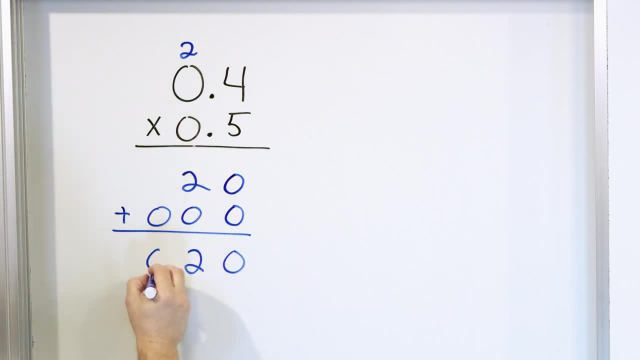 The 2 and the 0. give me a 2 and the 0 just goes right here. So you see, what we've done is completely ignore the decimal point. The decimal point is: we just pretend it's not there, right, And we get the. 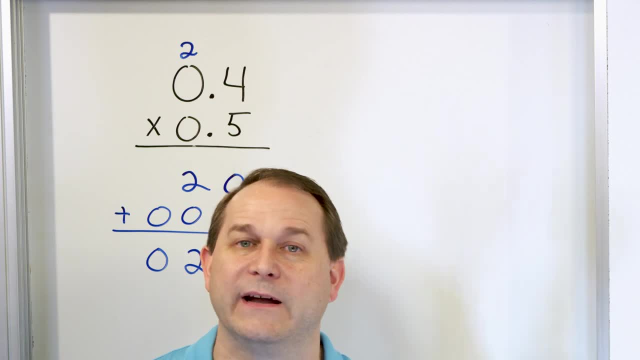 numbers in the answer, and then now I have to show you how to put the decimal in the final answer. What you do is you look back to your problem and you ask yourself: how many digits do I have after the decimal? Here I have a decimal point one digit after the decimal, and here I have a decimal point. 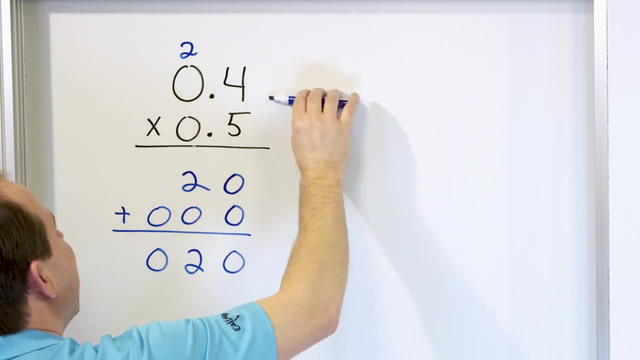 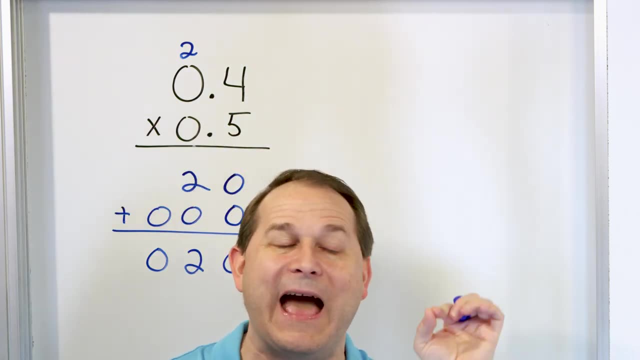 with another digit after a decimal. So for the whole problem, I'm going to put a decimal point in the answer. But the problem is I only have 2 digits after decimal points, One from here and one from here. So in my final answer I have to have 2 digits after the decimal point, One from here and 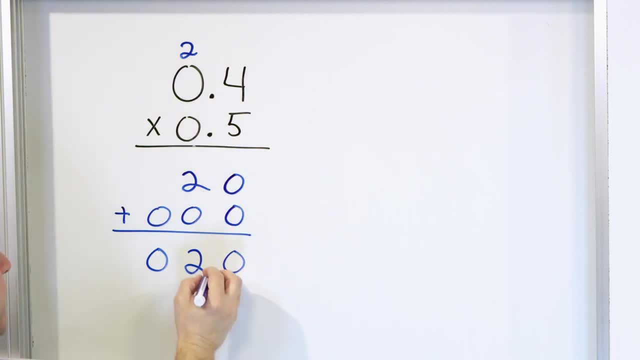 one from here, So I have to go. do I put it here? No, If I put it here, I'm only going to have one digit after the decimal, So I have to actually put it right here: 0.20.. 0.20 is the final answer. 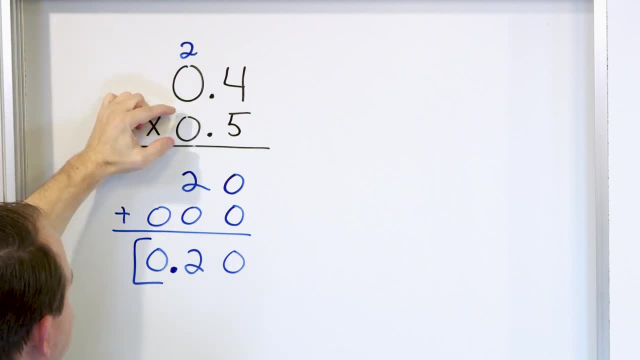 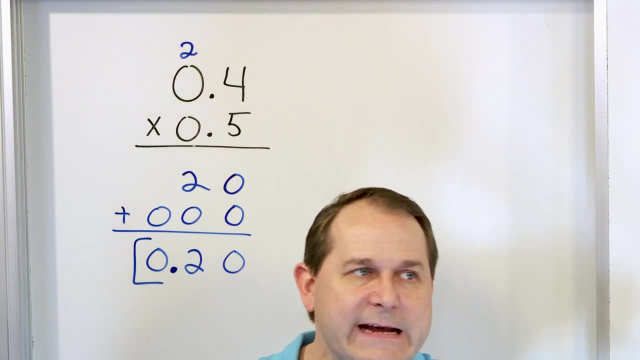 When you take 0.4 and cut it in half, which is what you're doing by multiplying by 0.5, the answer we we got from the pictures is 0.20. we did that by shading and chopping and counting and all that. 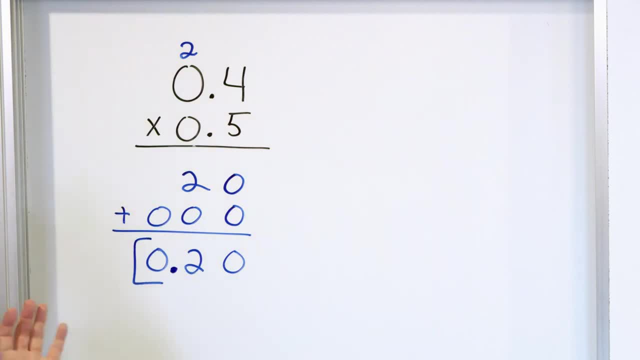 that was just for you to understand what's happening. and we now have put that aside and now we're calculating. and the way we calculate is: we do not. we the decimals just happen to line up here, but we do not have to line them up like this. we line the columns up, multiply as usual, pretend. 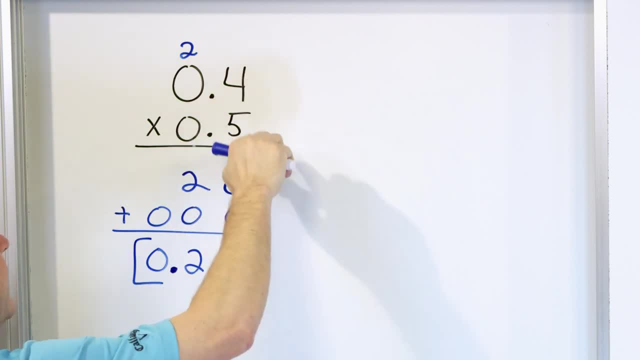 the decimals aren't even there. and then we have one digit after a decimal, here's another digit after a decimal, for a total of two. so the decimal must go here, so we have two digits after the decimal in our final answer. and notice that really, if you just cover up all everything four times, 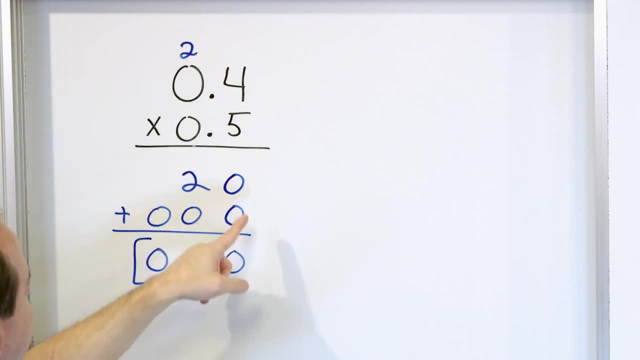 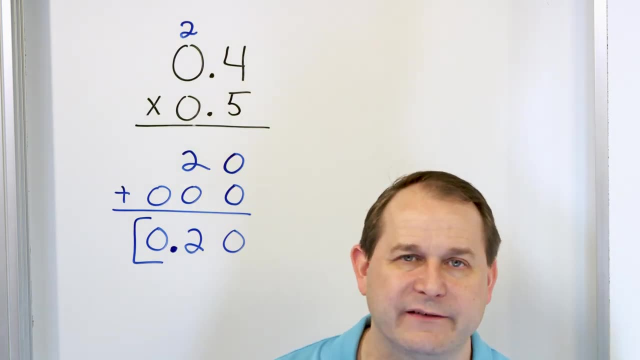 five. four times five is 20. here's your 20. we just have to put the decimal in the right spot. so really, when you're multiplying by decimals, it's like the decimals. they don't really affect the numbers of the answer, but the decimals in the problem tell you where the decimal point goes. 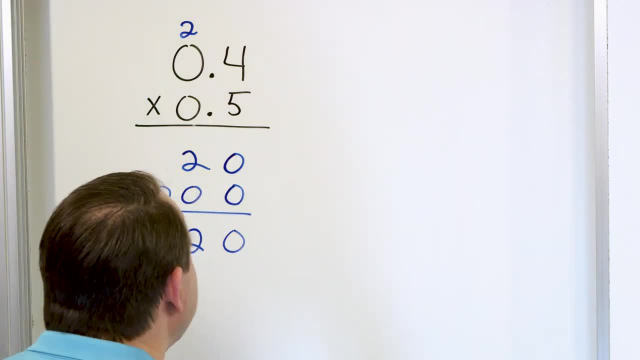 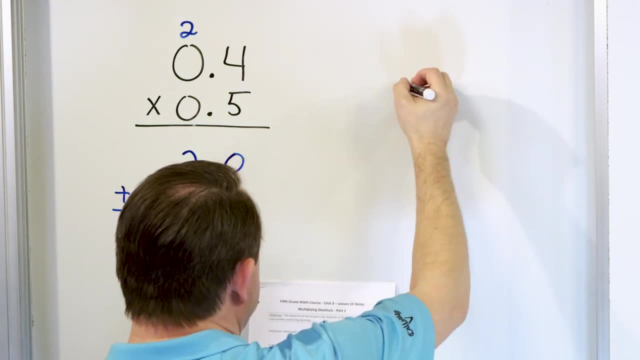 in your answer. that's what it does. now, instead of multiplying a decimal times a decimal, let's change things a little bit to something you know that. i think it's fairly easy for us to understand. let's say that i have the uh number 0.5 and we're going to 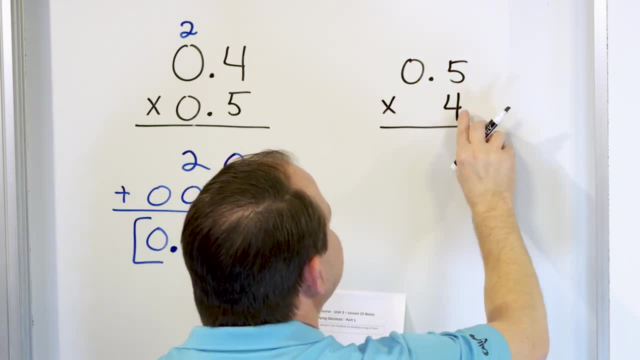 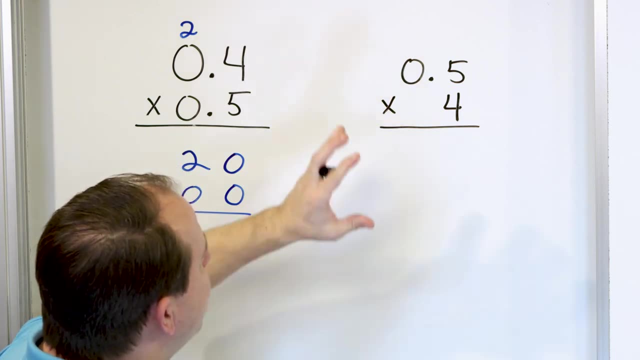 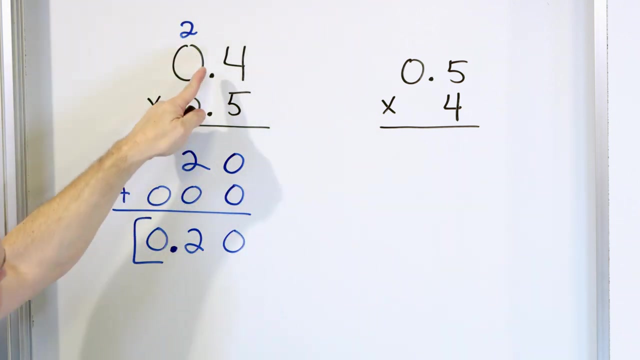 multiply it by 4. now notice the 4 has an invisible decimal at the end: 4.0, right, but i'm not lining up the decimals because i only line them up when i'm adding, when i'm multiplying. i don't need to line them up because the answer- the decimal point, does not just come down if it were to be a decimal point. 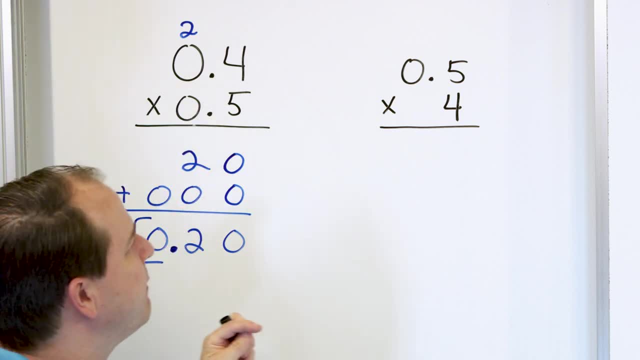 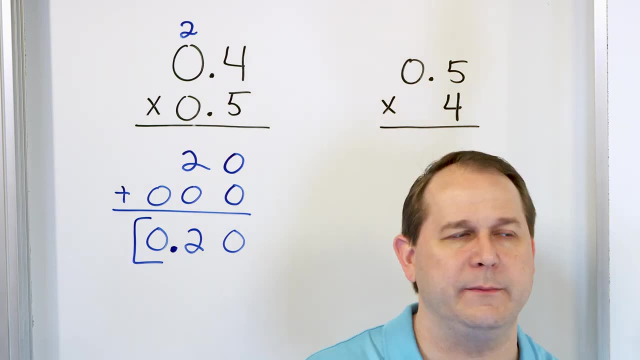 to come down, it would land here. i have to count decimals when we multiply, so here i'm not lining decimals up, i'm just putting things there. let's multiply, but let's also think. what do we think the answer is going to be: if i have four sandwiches and cut them in half by multiplying, i should only 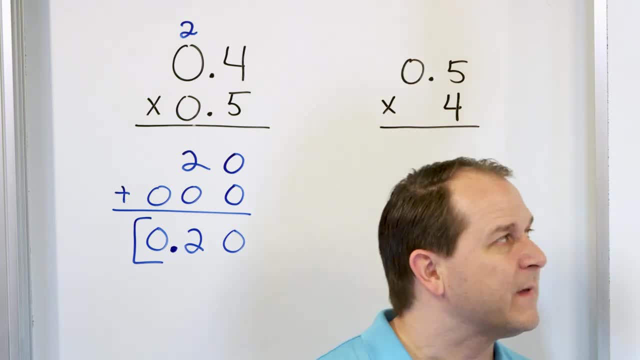 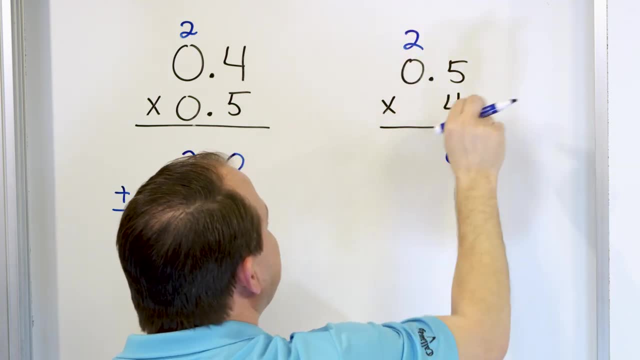 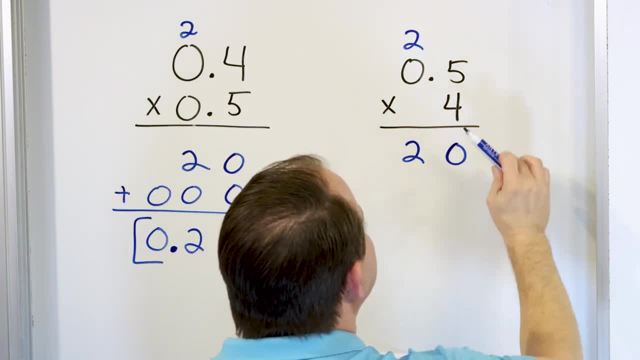 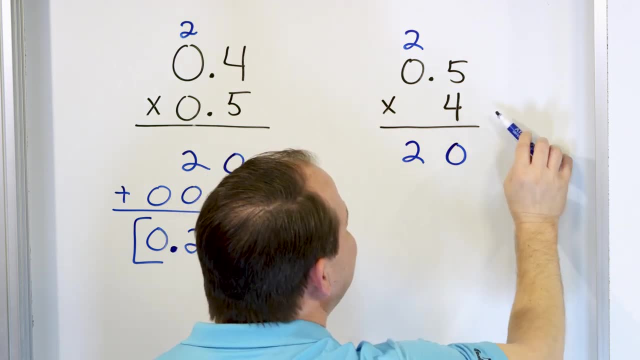 two. so here's our 20. now we look at our problem: how many digits after the decimal? here we have one. how many digits after the decimal? here there is no decimal point and there's no numbers after. so we don't have any uh digits after a decimal there at all. so in the problem we only have one digit. 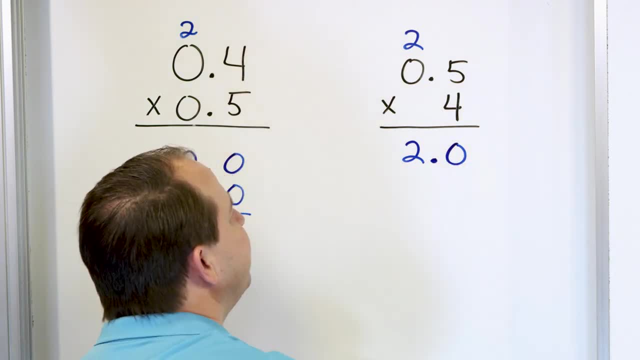 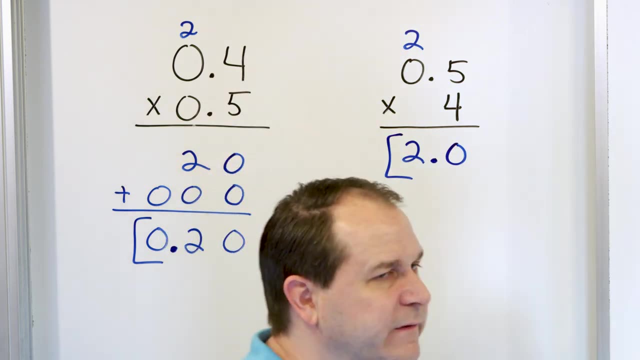 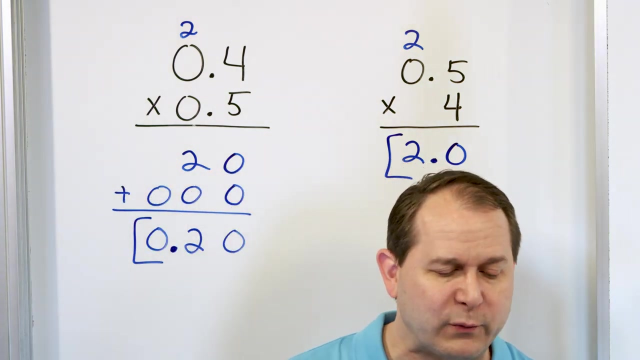 after the decimal. so in our answer we must have one digit after the decimal. so the answer to this would be 2.0. so if you have four sandwiches and you cut that in half by multiplying by 0.5, you should have two sandwiches left. that's exactly what this is: exactly two sandwiches left. so the rest of these problems. 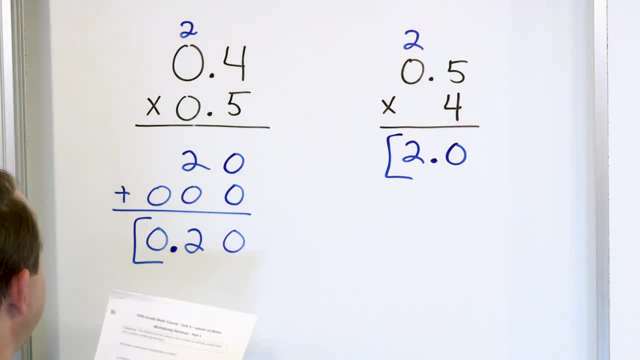 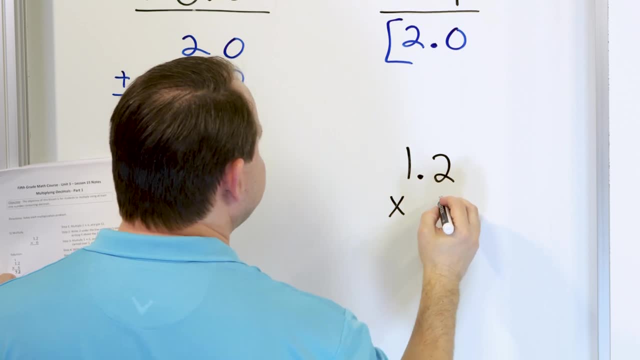 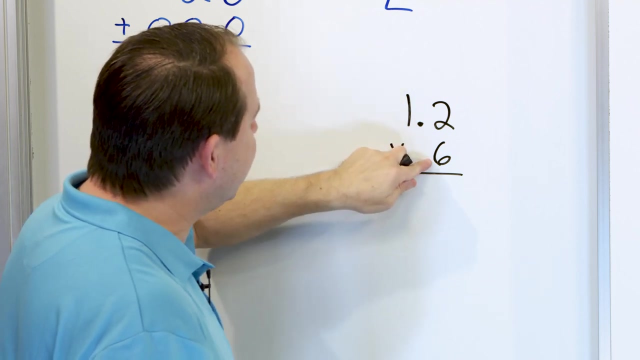 are going to behave the same way. we're going to write the problem down and we're going to solve it, uh, essentially by ignoring the decimal 1.2 times six. this is like taking a little bit more than a sandwich- 1.2 sandwiches- and multiplying six times, so making you know six copies and adding them. 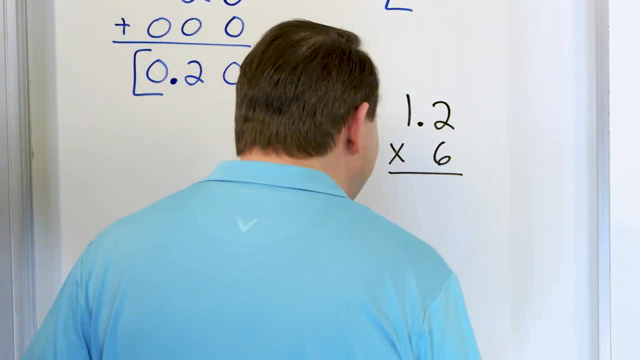 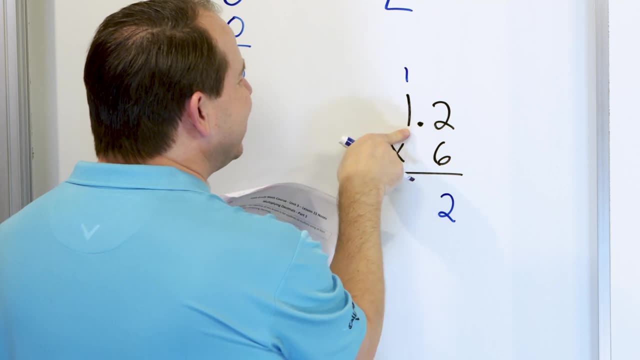 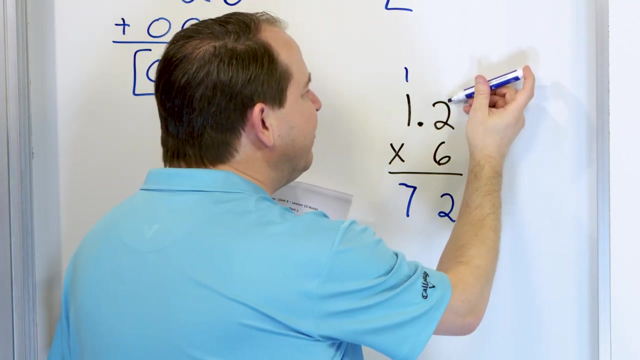 all together multiplying by six. we ignore the decimal, we pretend the decimal isn't even there. six times two is what twelve? so we put a two, carry a one. six times one is six. we add one more and we get seven. so those are our digits. that's it. now in our problem we only have one digit after a decimal. 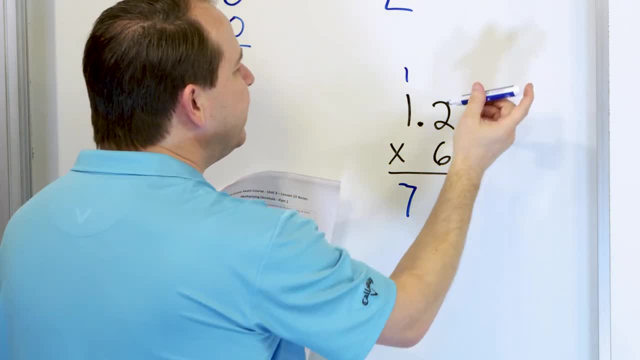 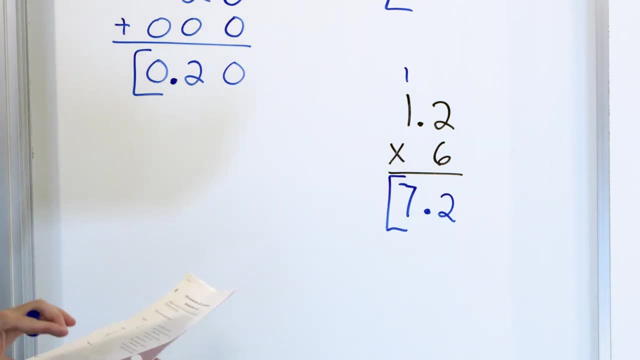 this one. we have no decimal, we have no numbers after, we only have one digit after a decimal. so it must go here, one digit after a decimal, for the answer to be 7.2. all right, 7.2. let's take a look at problem. 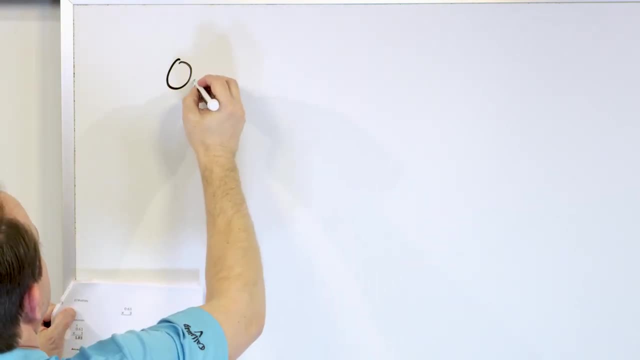 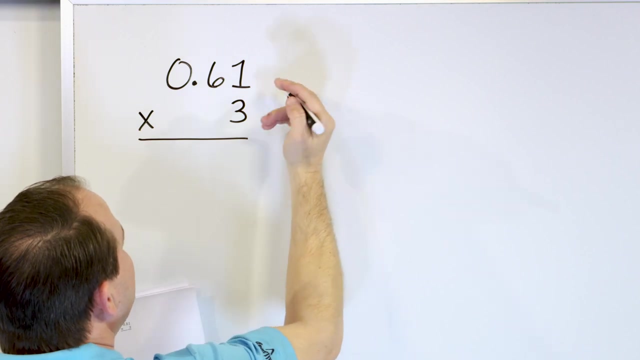 at the next problem. let's say we have 0.61 and we're going to multiply by three. again, i want to show you that there's an invisible decimal point. here we are did not line the decimals up. we did not line the decimals up here and we did not line the decimals up here. we do not do that for. 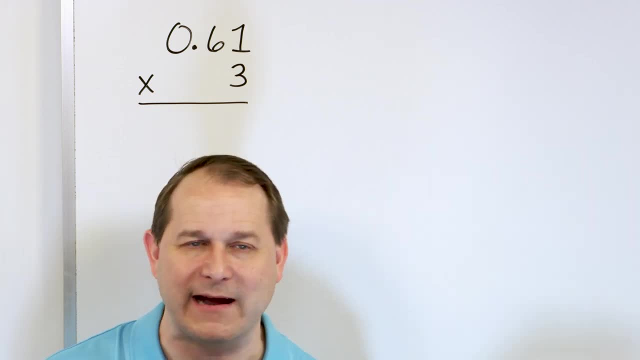 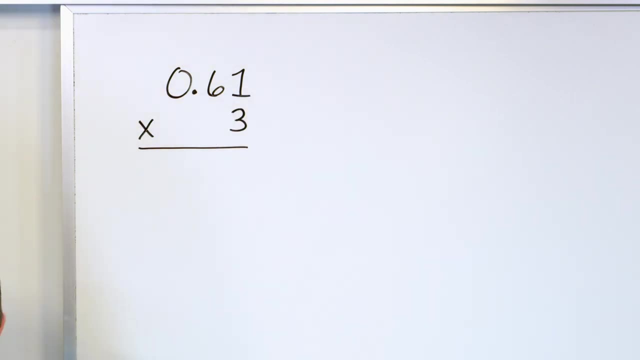 multiplying or dividing. we only do it for adding and subtracting. i know it's a little weird in the beginning, but you're going to have to get used to it. we push everything over, just like a regular multiplication problem. what is three times one, well, that's three. what is three times six, that's 18. so we put an eight, carry the. 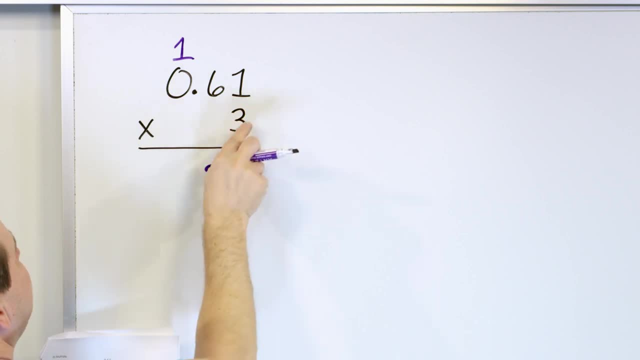 one. three times zero is three. one more, i'm sorry. three times zero is zero, any time. anything times zero is zero plus one is one. and now for the decimal point. we have two digits after a decimal. nothing here. so in our final answer we must have two digits after the decimal. the answer is 1.83. 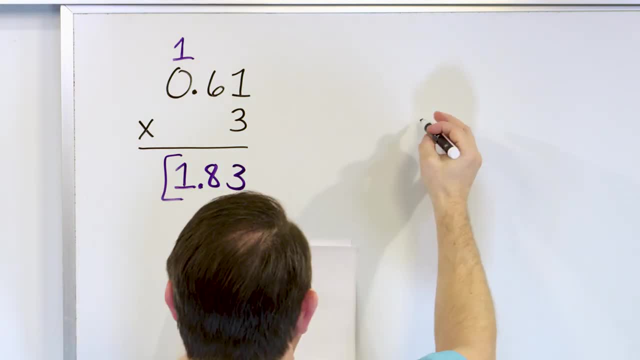 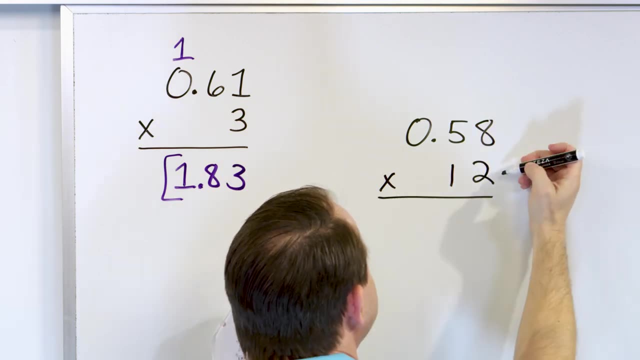 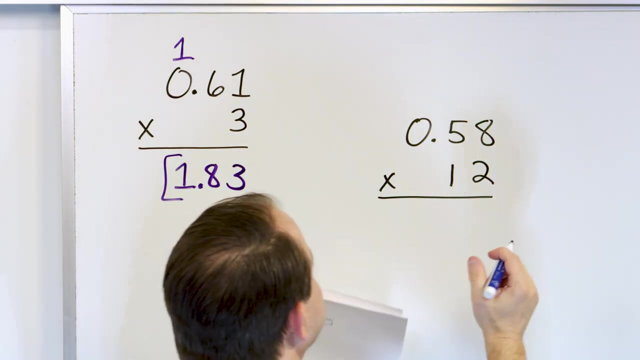 all right. next problem: let's say we have 0.58 and we're going to multiply. that times 12.. again, there's an invisible decimal after the 12. we have not lined it up with this. we just push the numbers over into the columns and we multiply. 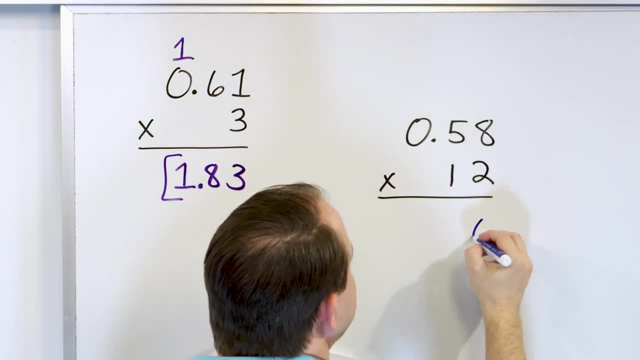 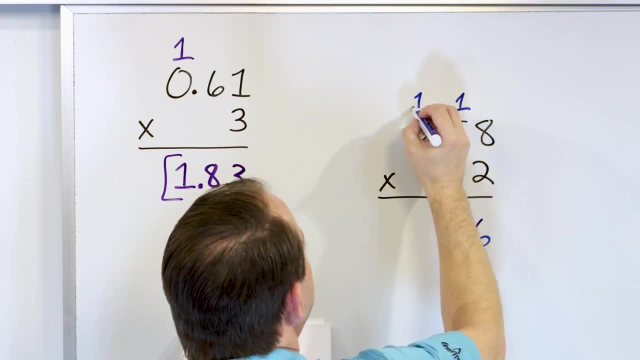 starting with the two. two times eight is what 16. so we put a six, carry a one five times two is what 10. one more is 11. so we have a one and we have to carry a one two times zero, zero. one more is one. 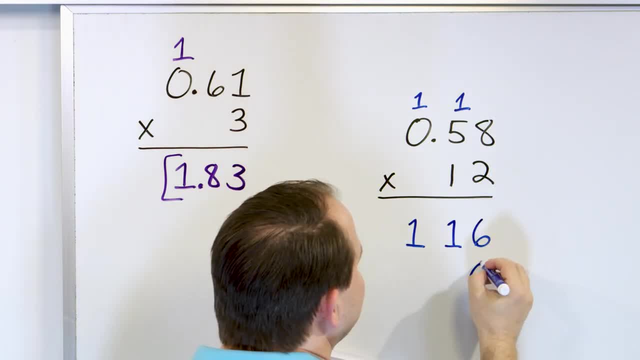 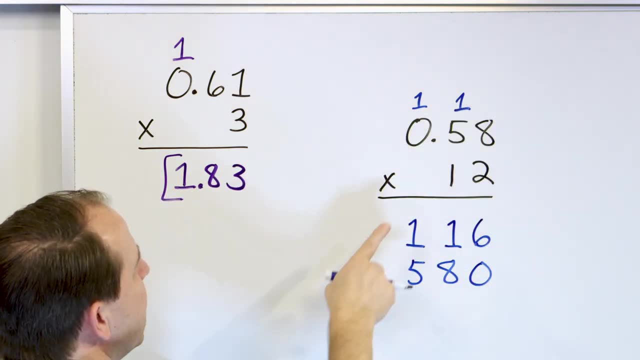 so we're done with that. now we have to multiply by the one, so we drop a zero. one times eight is eight. one times five is five. we don't have to add these. that's from the previous step. one times zero is zero, and then we add. what do we get for? 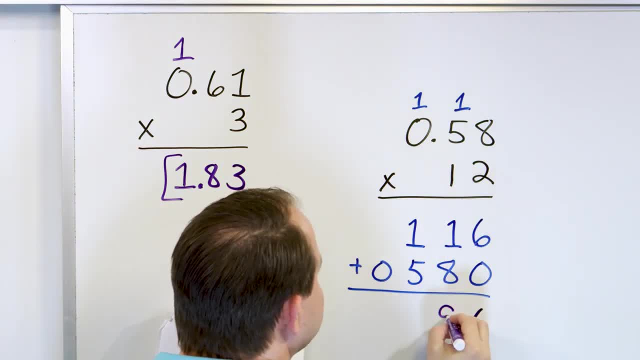 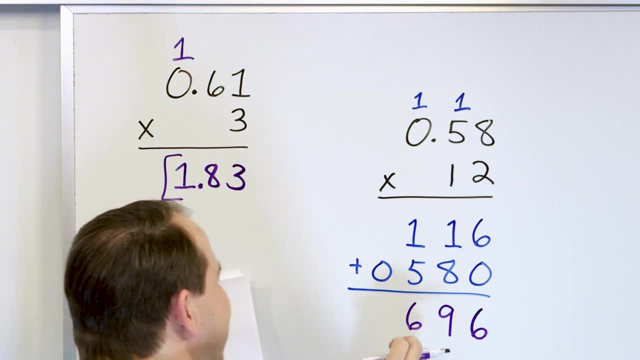 the answer six plus zero is six. eight plus one is nine. five plus one is six. and now we do have a zero plus a zero, but we don't really put leading zeros and numbers. so the answer is six, nine, six. but where does the decimal go? our problem has two digits after a decimal. 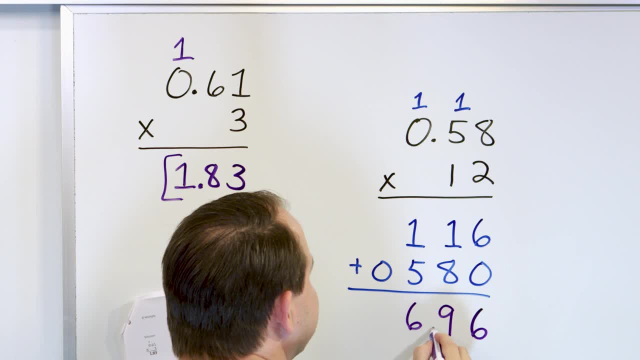 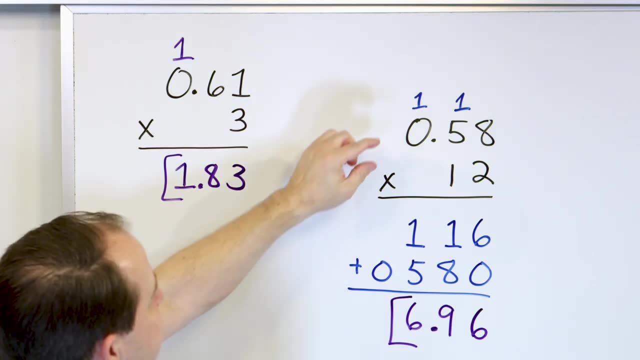 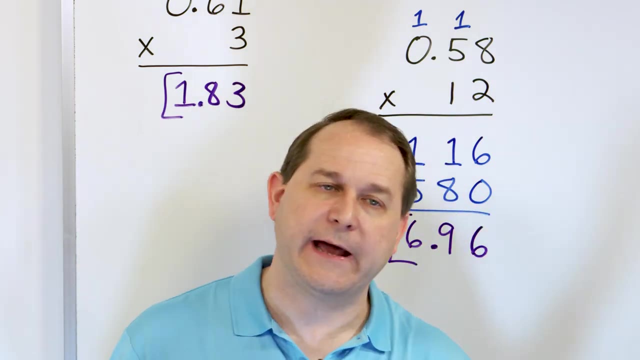 and then no digits after decimal, for a total of two. there must then be two digits after the decimal in our final answer, and then the answer is 6.96. so if i take 0.58, which is a little bit more than half of a sandwich, and i multiply that times 12 and add it all together, then i'm going to have 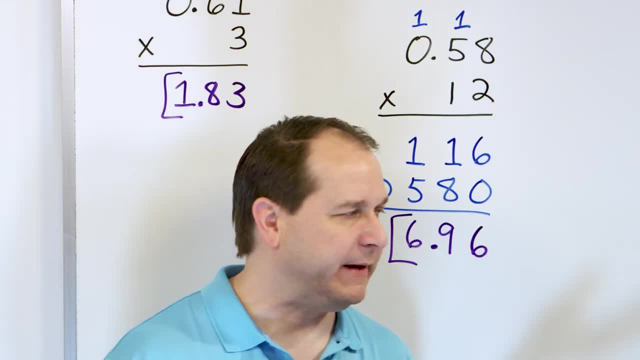 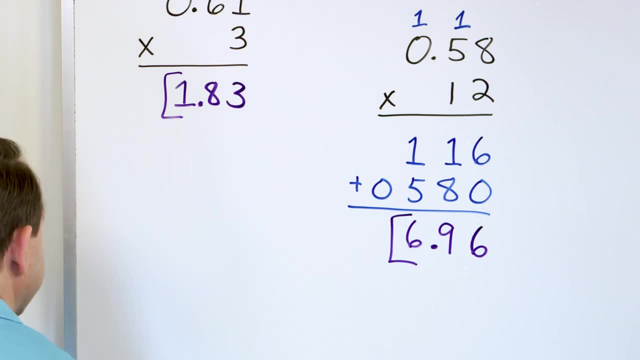 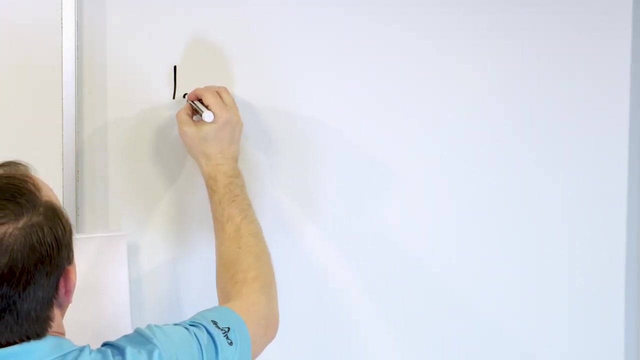 almost seven sandwiches. basically, that's what that really means: a little bit less than seven. 6.96 is a little bit less than seven. all right, let's take a look at the answer to this question, problem uh, number four. problem number four: let's say we have 1.21 and we're going to multiply that. 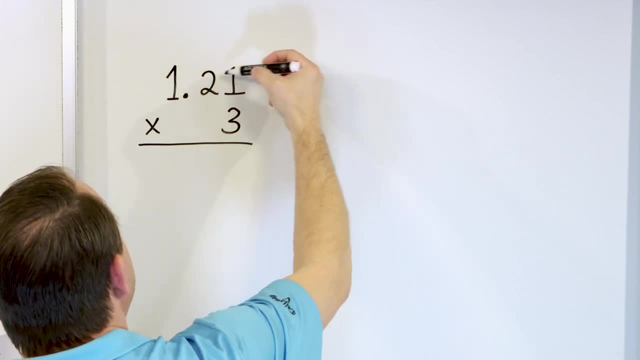 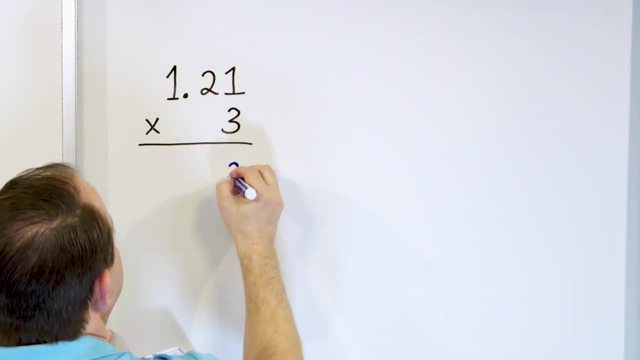 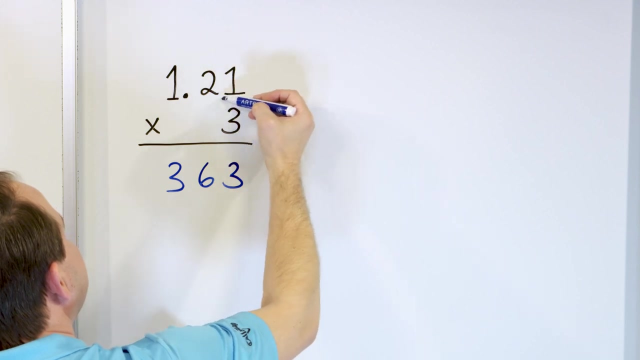 times three. so this means i have a little bit more than one sandwich- 1.21 sandwiches- and i'm going to triple it. what am i going to have in the end? three times one is what three. three times two is six. three times one is again three. and then for the decimal, i have two digits after the decimal here. 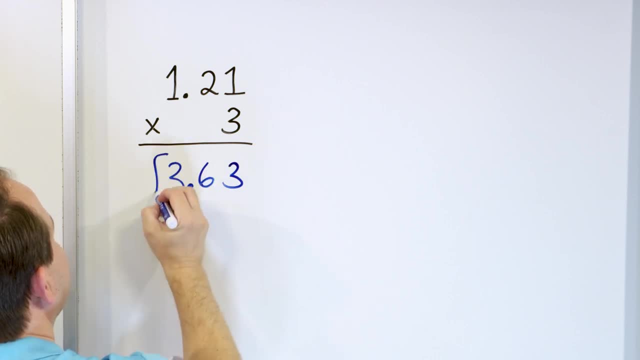 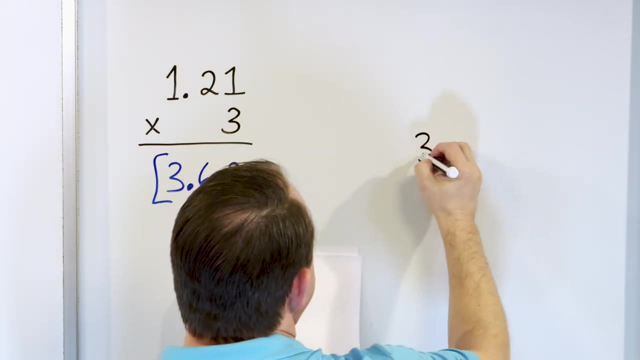 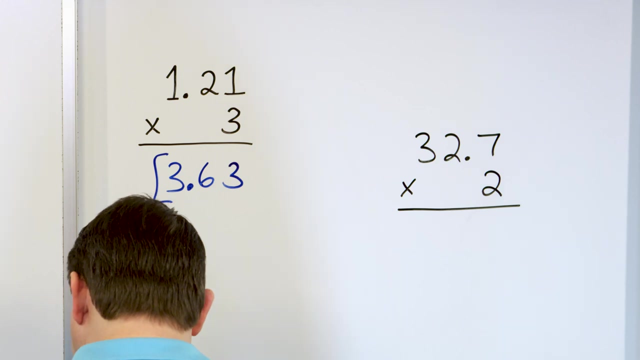 my answer must have two digits after the decimal, which means i go right here and the answer is 3.63. all right, here's the halfway mark. let's say we have 32.7 and we're going to multiply that times two, so basically we're going to double it. what do we have? seven times two is what 14 carry the one. 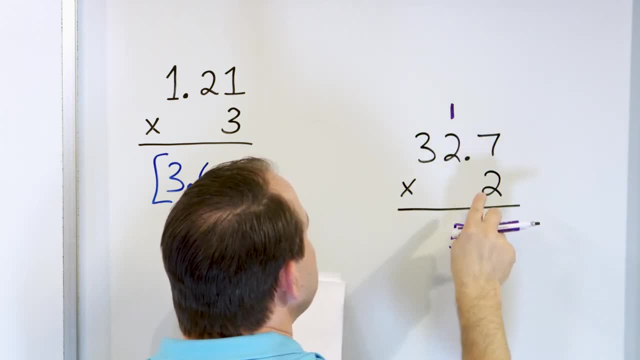 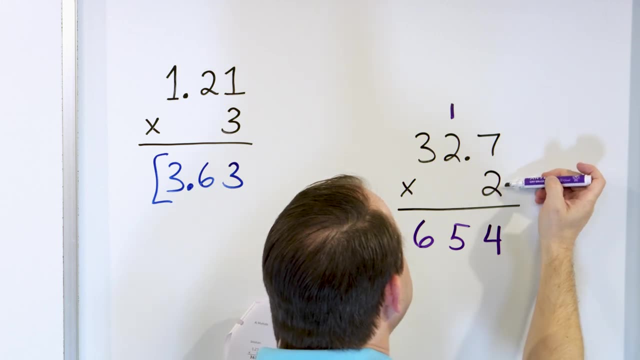 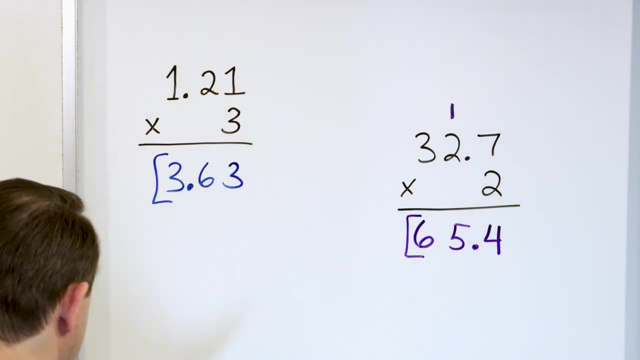 two times two is four. add one more, which is five. two times three is six. that's all the multiplying up, which is two is five. so that makes our decimal. we have one digit after the decimal and nothing here. so total: we have to have one digit after the the decimal point. for 65.4: 65.4. 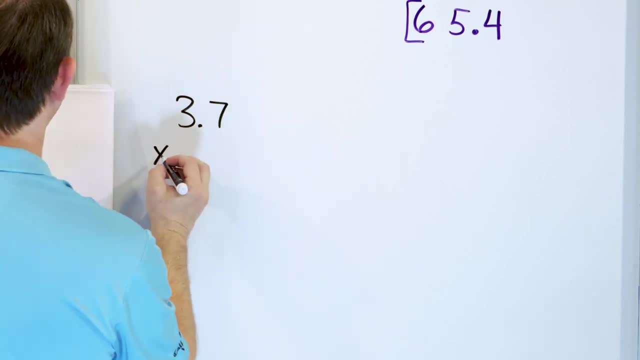 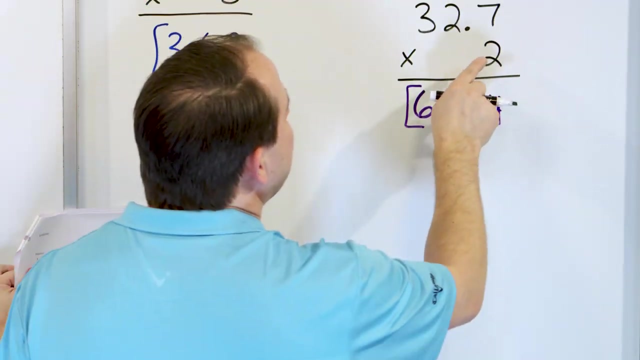 all right, let's take a look at 3.7 and we'll multiply that times 1.5. now notice, in this case the decimals are lined up, but that's not because i'm lining them up on purpose, it's because the where I have to have the columns lined up and so the decimals happen to be here. 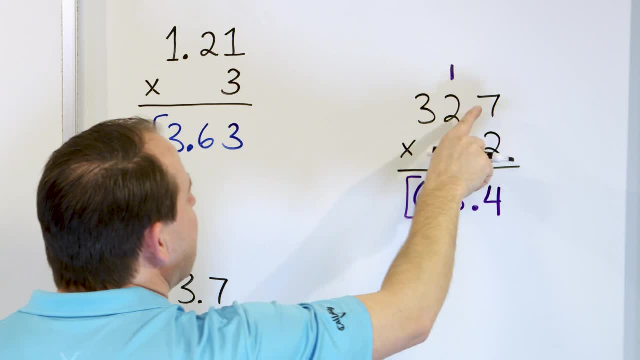 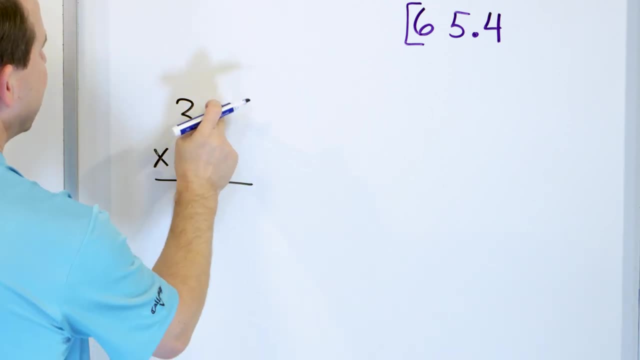 I push everything to the right. the columns are lined up. the decimals are not lined up in these problems. It's just a coincidence in this problem. So let's start by multiplying by 5.. 5 times 7 is what 35.. 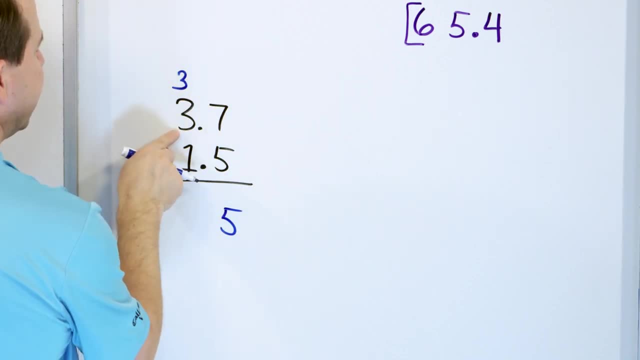 That means I put a 5 and I carry a 3.. 3 times 5 is 15.. Then we add 16,, 17,, 18.. So I have to put the 18 right here. Now we multiply by the 1.. First we have to drop a 0.. 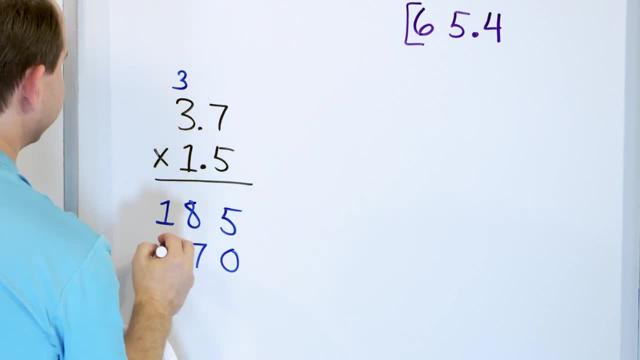 Then 1 times 7 is 7, and 1 times 3 is 3.. I don't add this because that was from before. Finally, we have to add these numbers: 5 plus 0 gives us 5.. 8, let's go up by 7.. 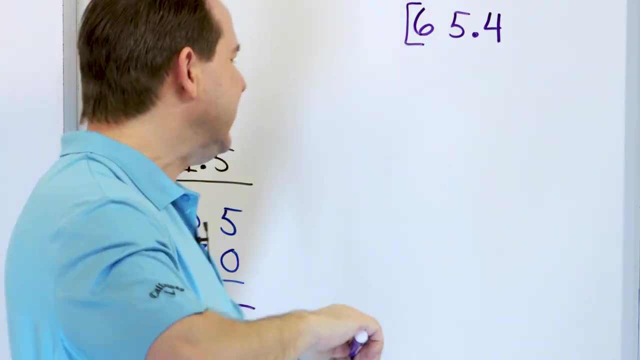 9,, 10,, 11,, 12,, 13,, 14,, 15.. We land on 15.. So we have to put a 5 here and we carry a 1 to the next column 3,, 4, 5 goes here. 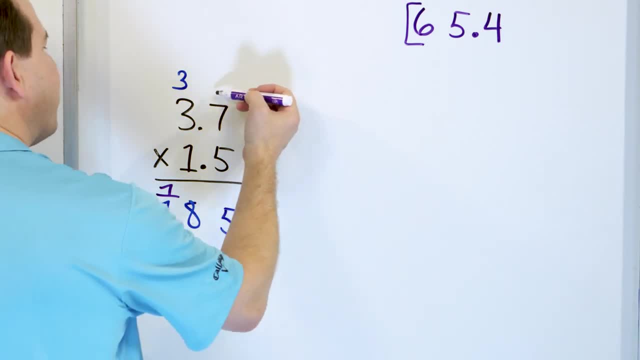 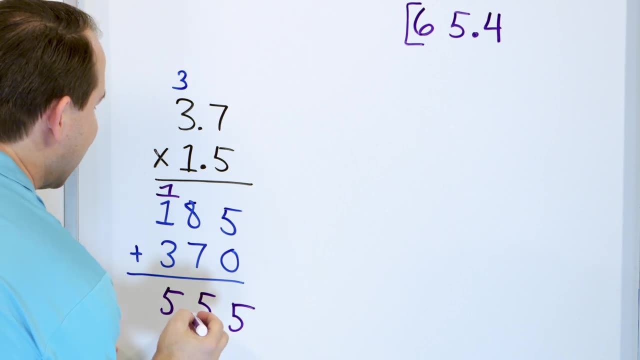 So we have 5,, 5,, 5.. Now where does the decimal go? In our problem? we have one digit after a decimal here and one digit after a decimal here, for a total of 2.. So then we have to have the decimal here. 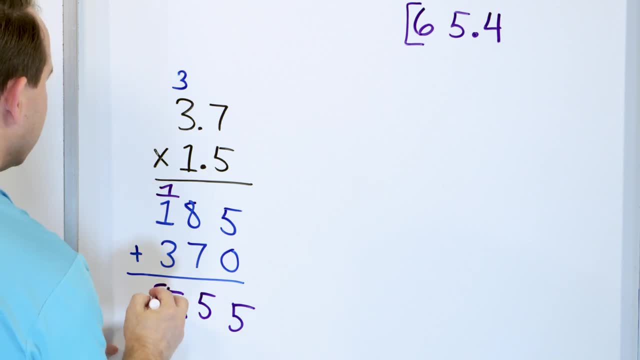 We have to have two digits after the decimal, One from here and one from here. Now it's important for you to realize that what we're doing is counting digits after the decimal and counting digits after the decimal. You might think that you just drop that decimal down. 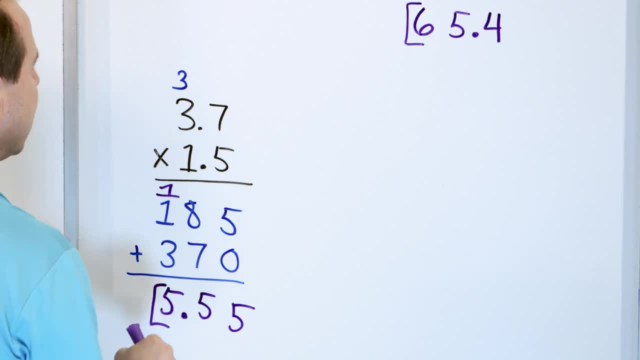 but if you just drop it down, you would probably think it lands here, So you can't just guess. You need to count. You need to count how many digits after the decimal and then put it in the proper location. All right, So let's take a look at our final four problems. 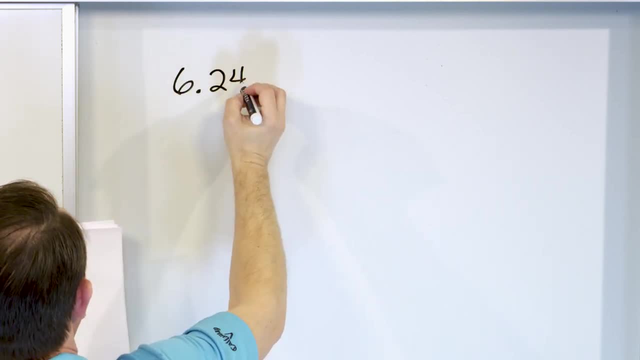 Let's take 6.24, and we'll multiply it times 2.8.. Notice that these decimals are not lined up The way I have it is: the columns are lined up with the numbers, but the decimal points are not, And that's the way we do multiplication. 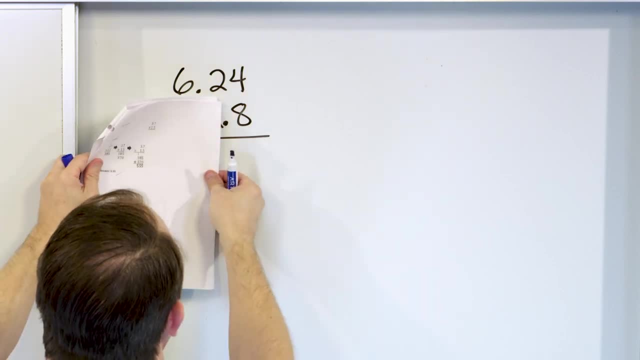 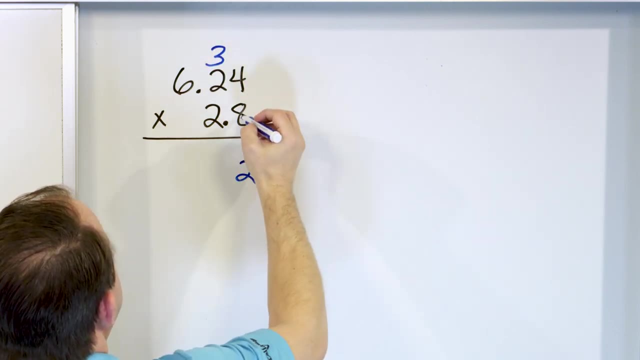 We don't line the decimals up. Start by ignoring the decimal Multiply by 8.. 8 times 4 is 32.. So we put a 2 here, Carry a 3. 8 times 2 is 16.. Going up. 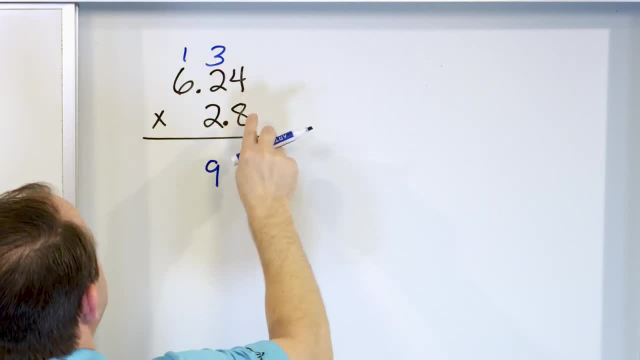 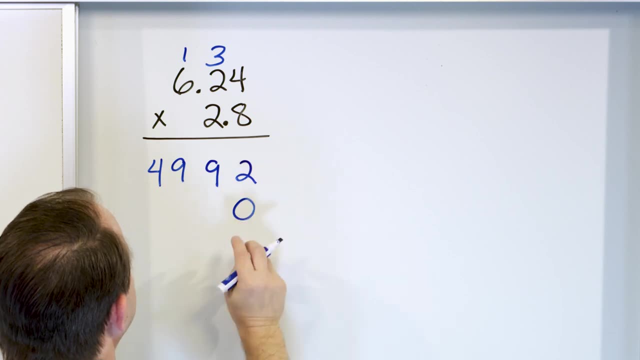 17,, 18,, 19.. We put a 9.. Carry a 1.. 8 times 6 is 48.. One more is 49. So we put the 49 down here. Now we multiply by the 2,, so drop a 0.. 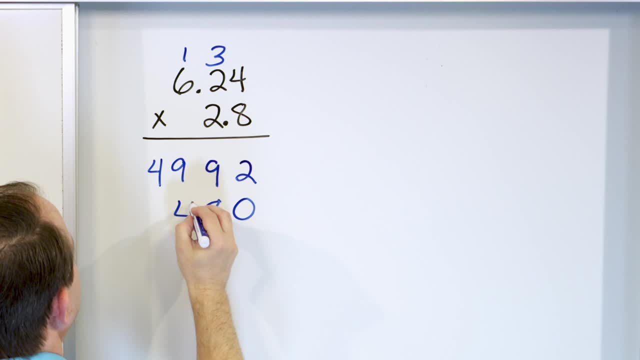 2 times 4 is 8.. 2 times 2 is 4.. We don't add these because that's from the previous step. 2 times 6. 6 is 12.. And then we have to add these numbers together. 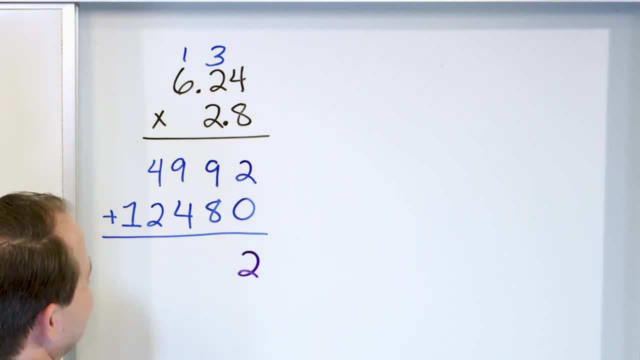 So the 2 comes straight down. 9 plus 8 is 17,, because 10 plus 8 is 18.. So 9 plus 8 is 17.. Carry the 1. This makes 10 plus the 4 is 14.. 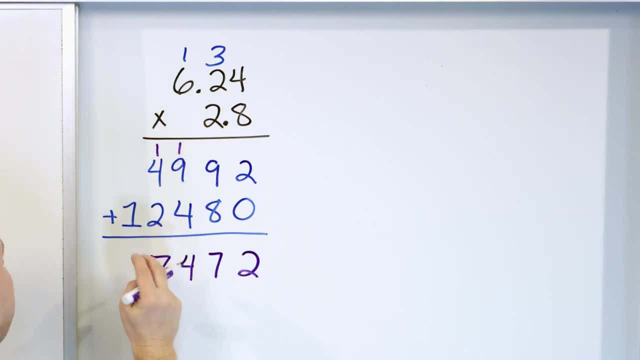 Carry. the 1.. 4,, 5,, 6,, 7 goes right here, And then a 1 drops down here. Now look at all these numbers. Where does the decimal go? It certainly isn't in a line, so we can't drop it down. 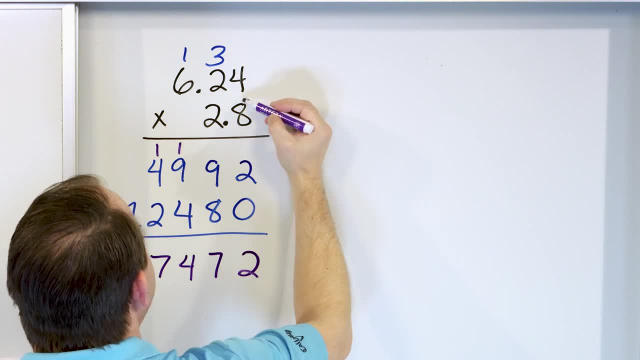 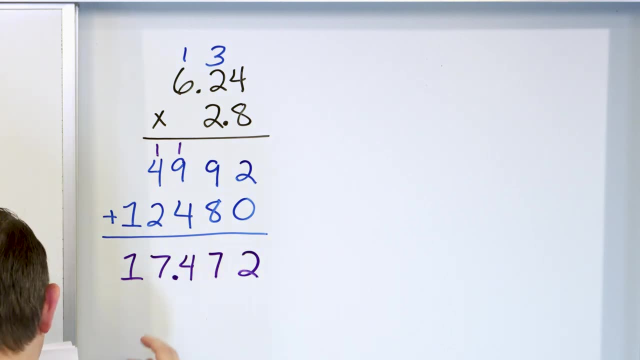 What do we do? We have 2. We have 2 digits from after the decimal here and we have 1 digit after the decimal here, for a total of 3 digits after the decimal. So in our problem we must have in the answer 3 digits after the decimal. 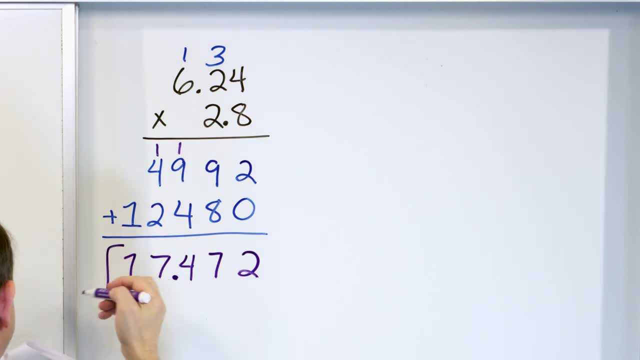 So the answer is 17.472.. Now we have not actually covered decimal positions past the hundredths place yet, but really it's the same thing, It's the same concept. Here is the tenths place, Here is the hundredths place. 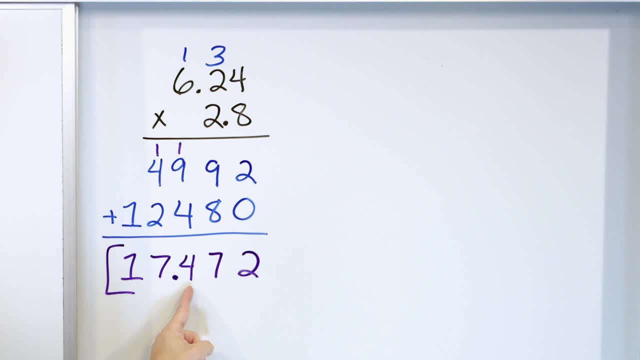 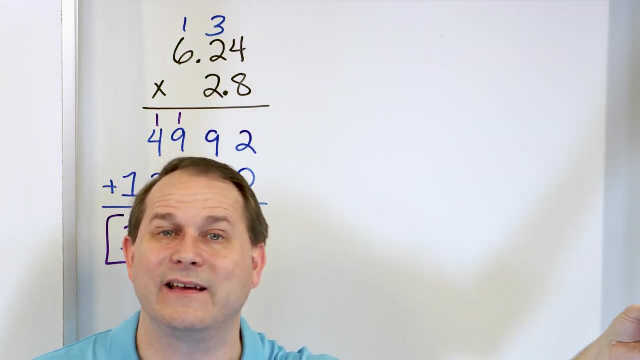 Here is the thousandths place. So what this means is: this digit is worth one tenth, Every digit here is worth one one hundredth, And every digit here is worth one one thousandth. It's worth a really tiny amount. The farther you go after the decimal, the digits mean less and less and less and less. 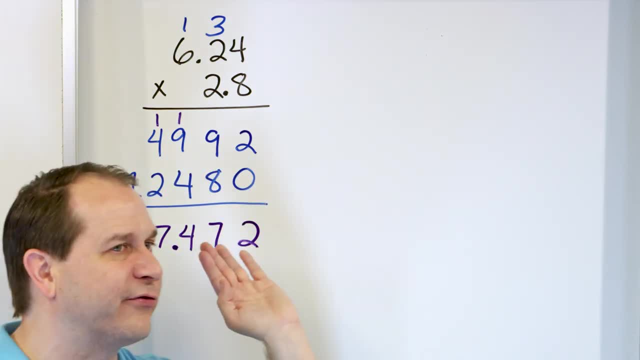 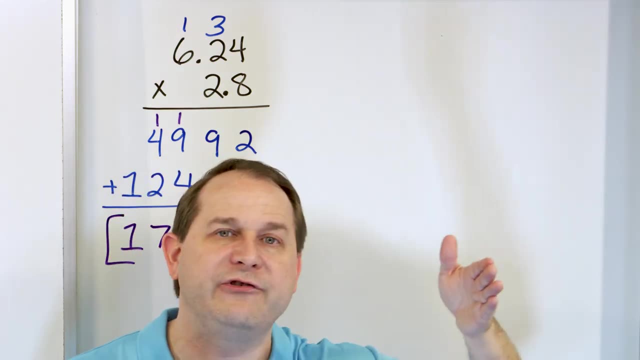 So in real life sometimes we either round the numbers or we just throw the last few numbers away because they don't matter. You can have numbers after the decimal that go on and on and on forever and those digits weigh us down But at the end don't really mean very much because they're only worth maybe one, one millionth. 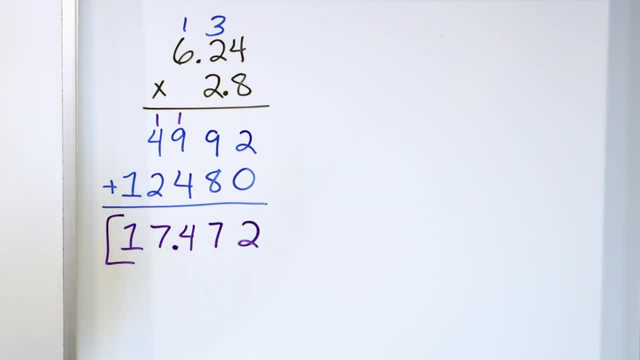 or one one hundred millionth or something like this. So don't stress out if you have a lot of extra digits. It looks like it's a big number, but it's really telling you have 17 whole pieces And then this represents how close I am to the next whole. 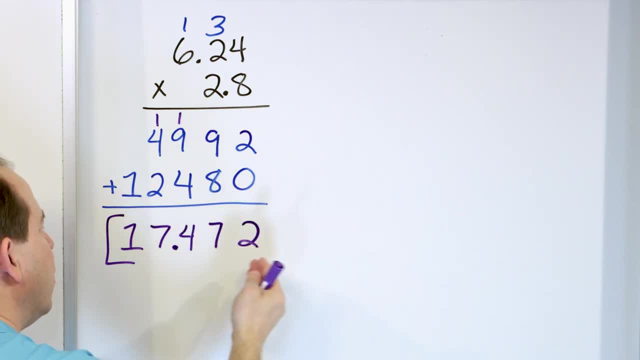 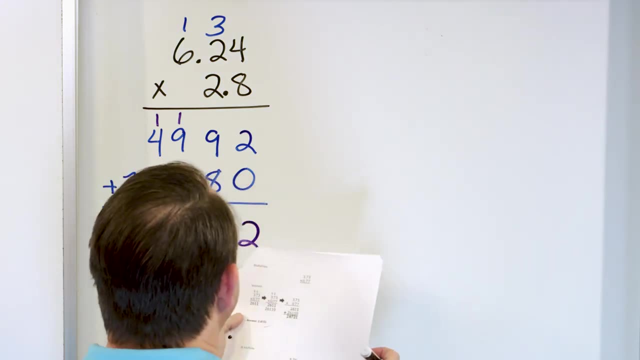 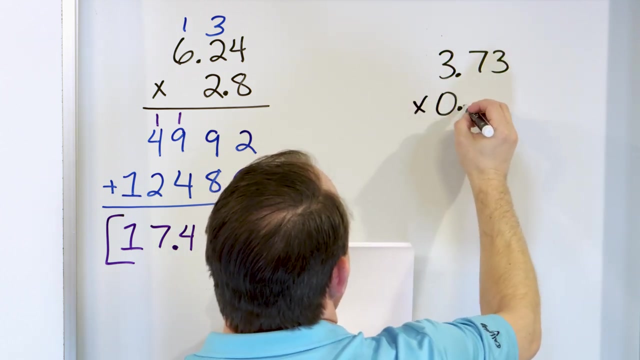 If I get to 999 after the decimal, then I'll roll over to 18, the next whole number. So 17.472 is the final answer. All right, Next problem: We're going to look at 3.73 and we're going to multiply that by 0.77.. 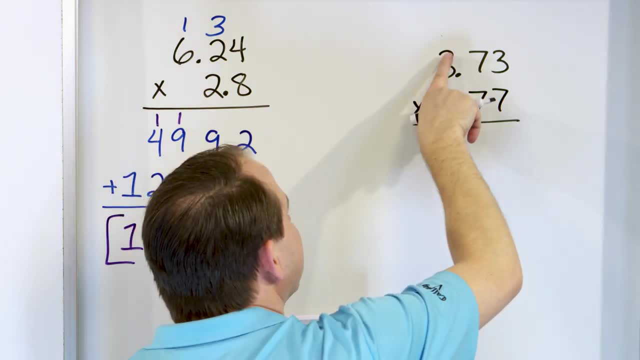 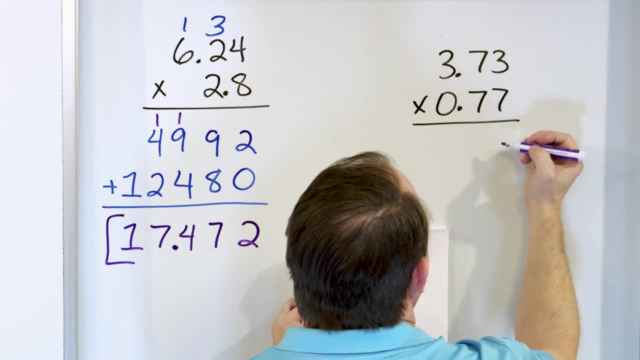 Now again, I'm not lining up the decimals. They only are lined up just because the columns are lined up with the numbers, All right. So what do I do? I say 7 times 3, I start here: 7 times 3,, 21.. 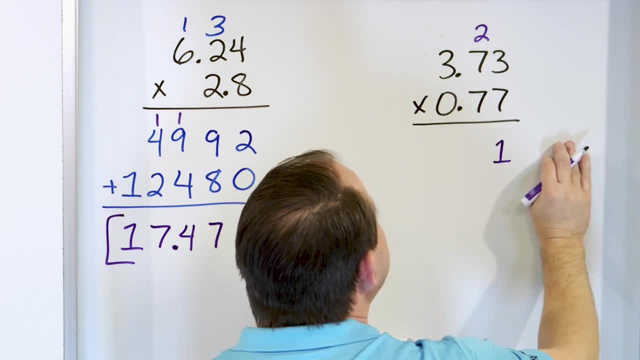 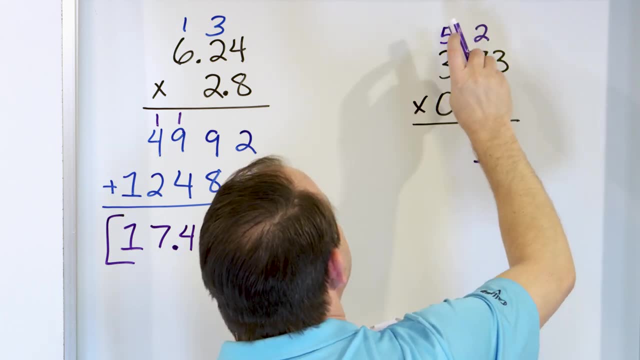 So I put a 1,, carry a 2.. 7 times 7, 49.. Go up 50,, 51.. Carry the 5. 7 times 3, 21.. Carry the 5. 7 times 3, 21.. 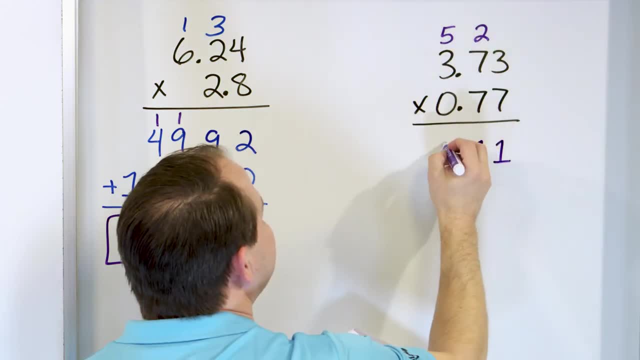 We go up 22,, 23,, 24,, 25,, 26.. 26 means I just put a 26 down here. All right, Now I've got to multiply by this 7, so I have to drop a 0.. 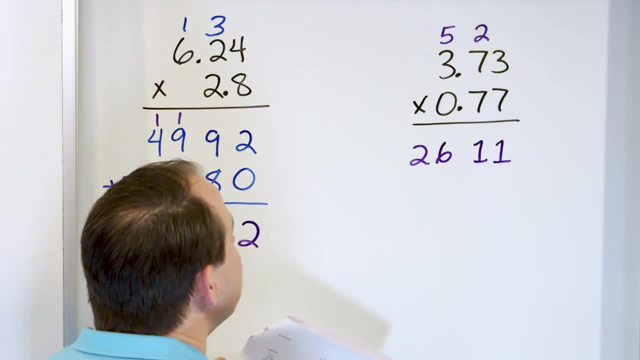 Again, 7 times 3 is 21.. So let me switch, probably switch colors. 7 times 3 is 21.. So again, I'm going to carry a 2.. 7 times 7 is 49. Then 50,, 51.. 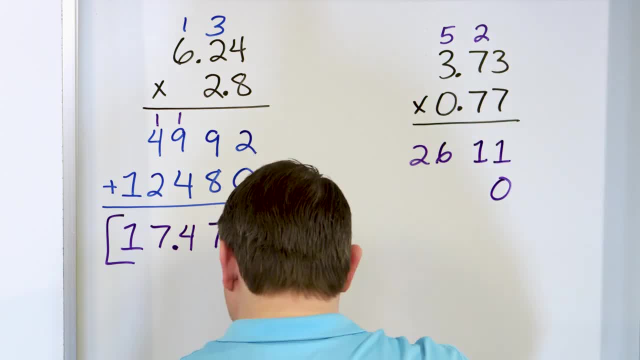 Carry the 5. And then 7 times 3 is 21.. Then we have 22,, 23,, 24,, 25,, 26.. So again, I'm going to carry a 2.. 7 times 7 is 49.. 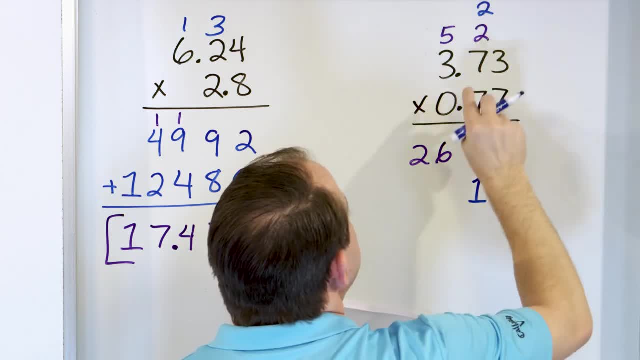 Then 50,, 51. Carry the 5. And then 7 times 3 is 21.. Then we have 22,, 23,, 24,, 25,, 26. So again, I'm going to carry a 2.. 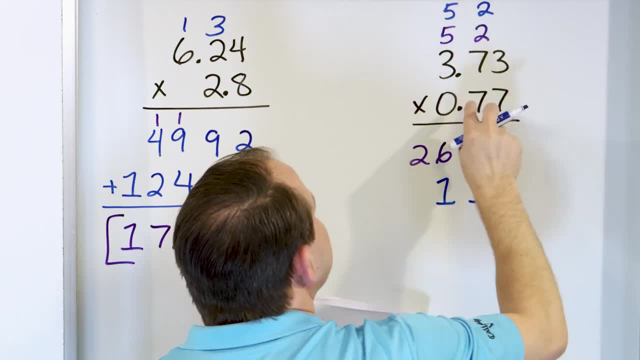 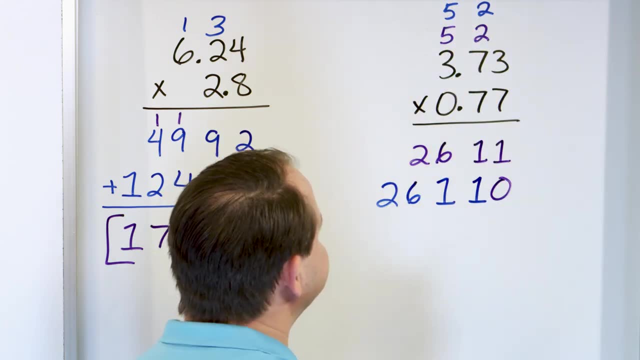 7 times 7 is 49. Then 50,, 51. Carry the 5. And then 7 times 3 is 21. Then we have 22,, 23,, 24,, 25,, 26. Put the 26 right here. 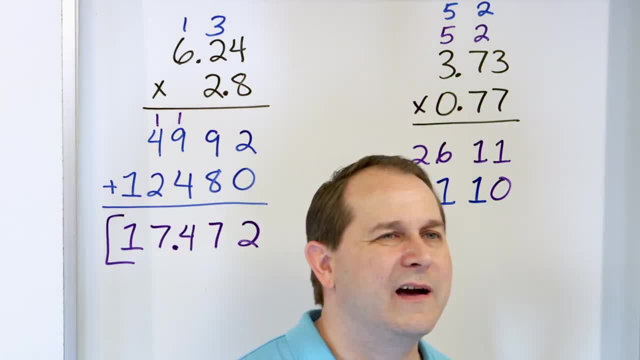 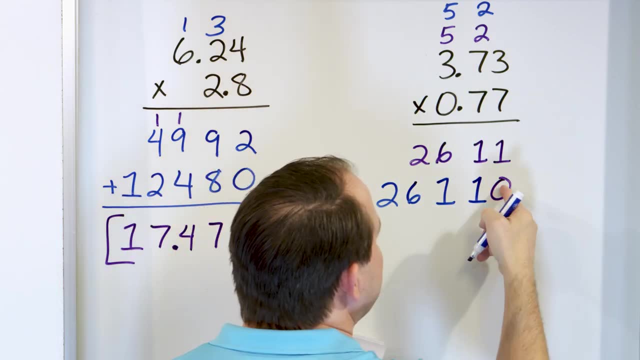 So I'm done multiplying by these. Now I do have another digit there, but multiplying by 0 doesn't do anything. Let's go ahead and do it, but you'll just see. If we're going to multiply by this digit, we have to not only add one, 0, we have to. 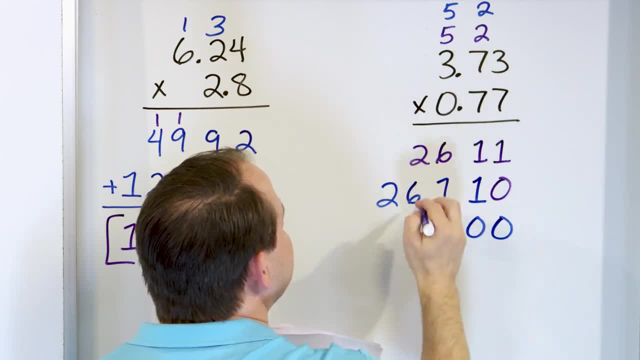 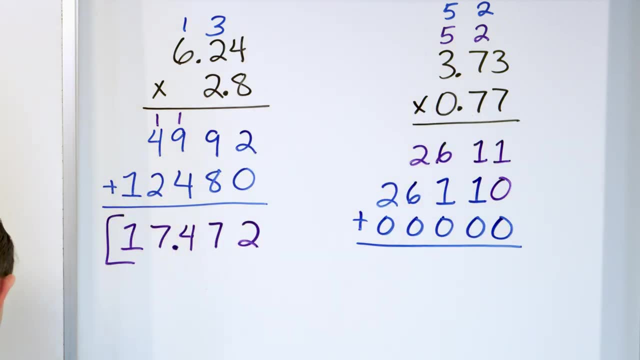 drop two 0s, Then 0 times. this is 0.. 0 times. this is 0.. 0 times, this Is 0.. So a leading 0 like that before the decimal doesn't change anything. The 1 drops down. 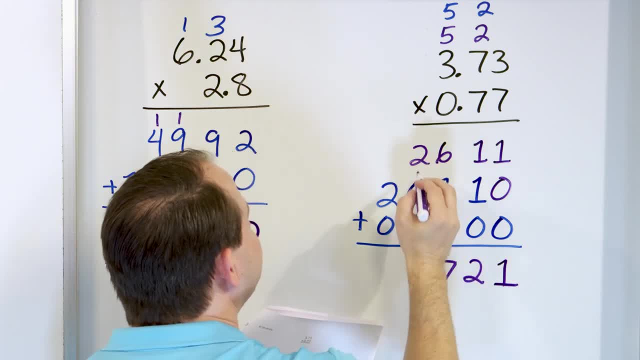 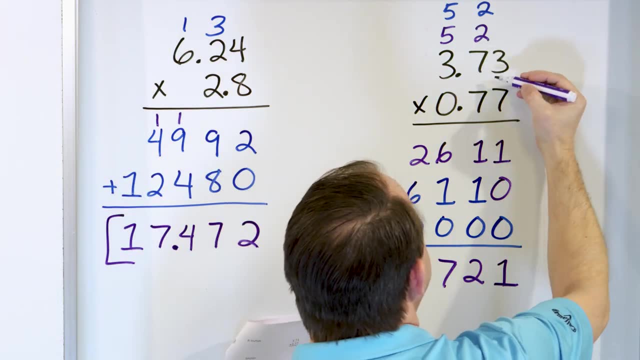 1 plus 1 is 2.. 6 plus 1 is 7.. 6 plus 2 is 8. And 2 drops down. Where does the decimal go? I have two digits here and two digits here after the decimal, for a total of 4.. 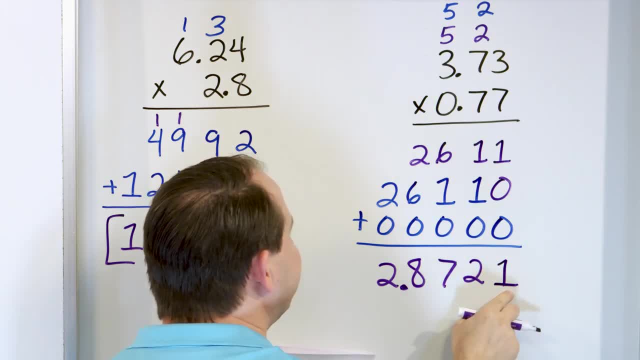 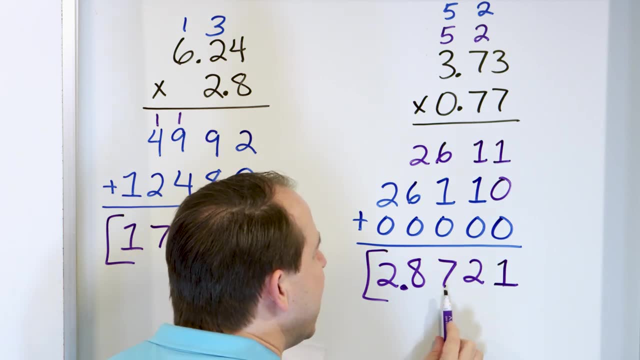 So I have to put the decimal right here: 1,, 2,, 3,, 4 digits should come after the decimal 2.8721.. So So this is the tenths place. This is the hundredths place. 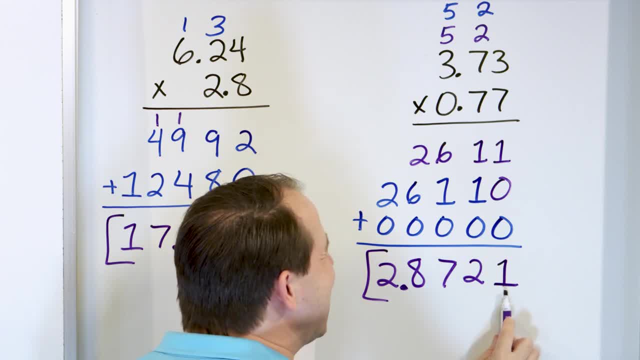 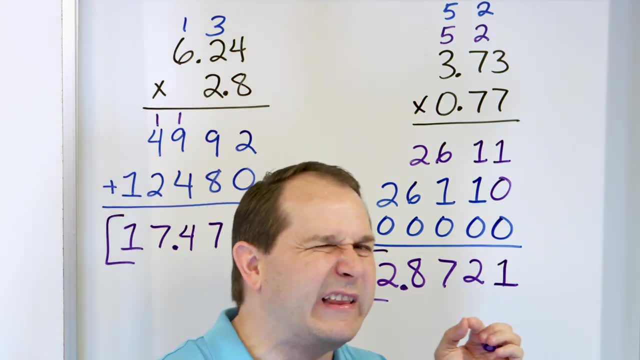 This is the thousandths place. This is called the ten thousandths place. It's worth even less, 10 times less, than what has come before it. So this one here has very little meaning in the number. It doesn't change the value of the number much, because the farther you go off to the 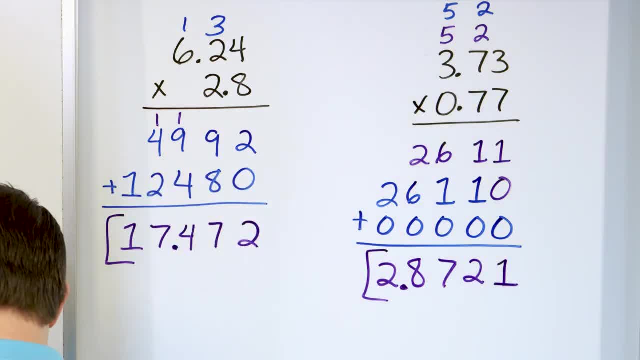 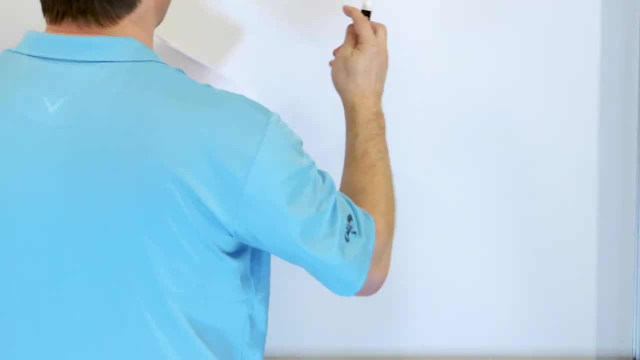 right after the decimal, the less and less the numbers mean. Okay, We only have two more problems. Okay, And we're going to conquer the next to last one right here. What about 4.36?? And we'll multiply it by 2.94.. 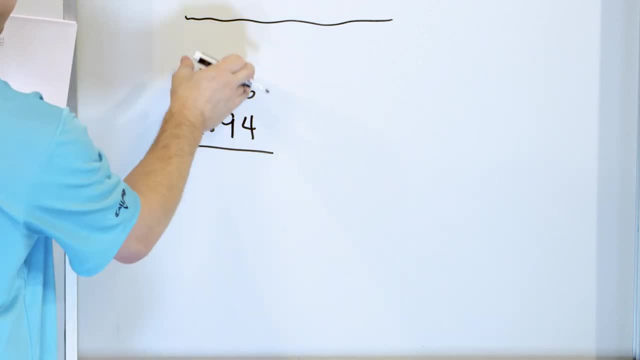 Again, I'm not lining up decimals, I'm just lining up columns and the decimals happen to line up. So this is going to be a big multiplication problem. First we have to multiply by 4.. 4 times 6 is 24.. 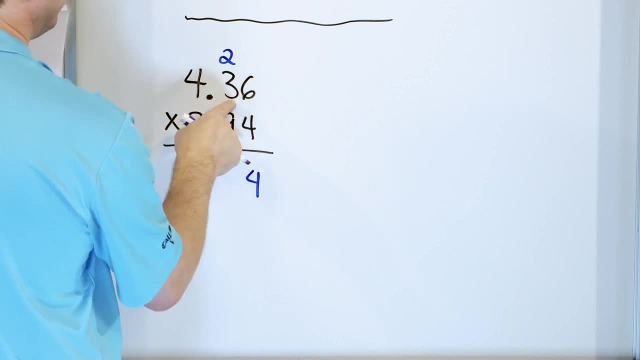 Carry the 2.. All right, 3 times 4 is 12.. Then we go up 13,, 14.. Put a 4 in there. Put a 4, carry the 1.. 4 times 4 is 16.. 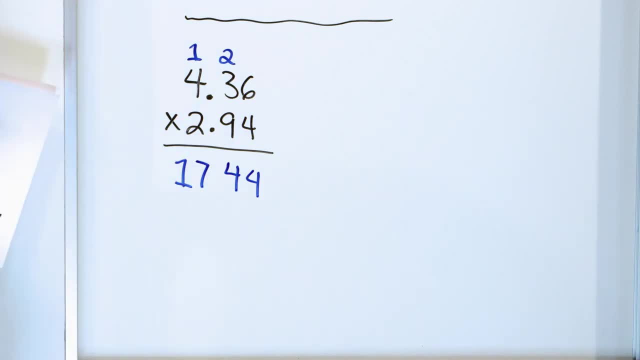 One more makes 17.. So the 17 goes there. Now we're done with the 4.. Now we multiply times 9 and we have to drop a 0., 9 times 6, 54.. Let me switch colors. 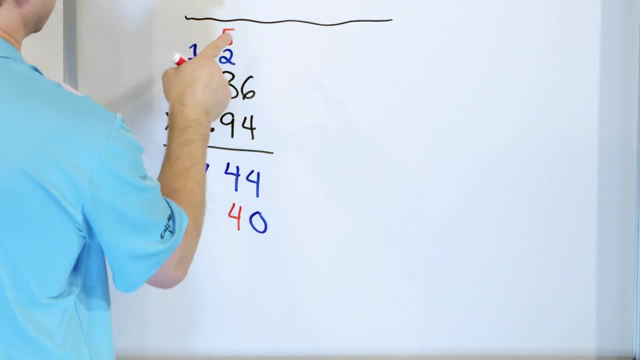 54. Put a 4, carry the 5 to the next column here 9 times 3, 27.. We add 28,, 29,, 30,, 31,, 32.. 32 means we carry a 3.. 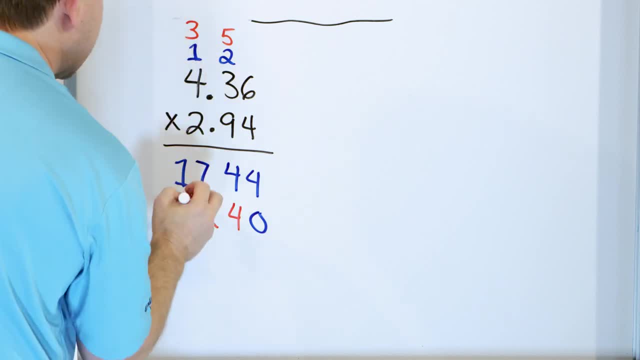 9 times 4, 36. Then we add 37,, 38,, 39. And 39 goes right there. Now we're done with that. Now we have to multiply times the 2.. So I think what I'll do is I'll go to purple here. 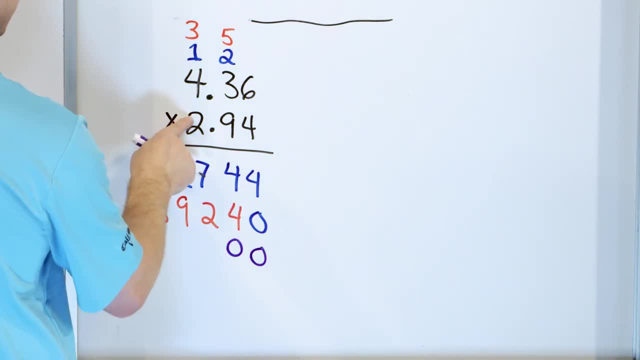 We have to drop two 0s in this guy right here. Multiply by 2. 2 times 6 is 12.. Carry the 1. 2 times 3 is 6.. That just goes right here. Actually, 2 times 3 is 6.. 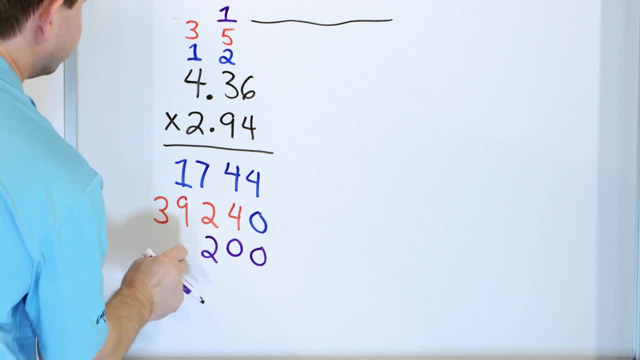 We have to add the 1.. Right, We almost made a mistake there. It has to be a 7.. Like this, All right. And then 2 times 4 is 8.. We don't have to add any of those other numbers. 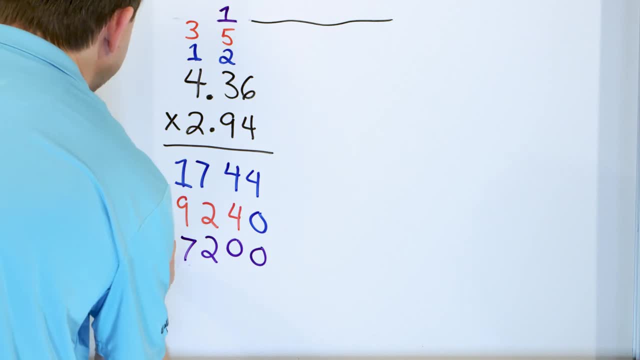 That's from before. So 8,, 7, 2,, 0, 0.. Now we add all of these numbers together, What are we going to get? We'll go back to black. The 4 just drops right on down. 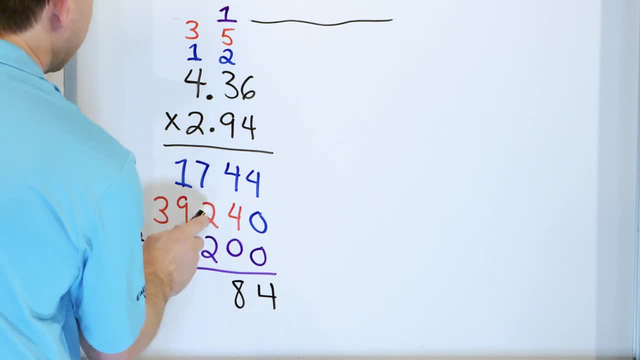 4 plus 4 is 8.. That goes right here: 7,, 8,, 9,, 10,, 11.. We have to carry a 1.. Barely enough room right there to carry a 1.. 9 plus 1 is 10.. 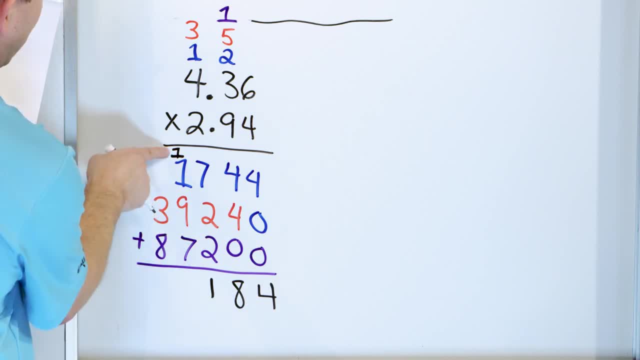 This is 10.. This is 10 plus 7,, 17. So we have 17.. One more is 18.. Put an 8. Carry the 1 up here: 8,, 9,, 10,, 11,, 12.. 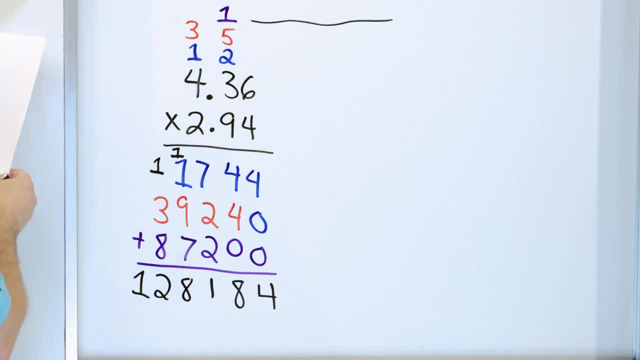 So we have 12.. We have a 2 here and we have a 1 here. So 1, 2, 8,, 1, 8, 4.. Now we have to figure out where does the decimal go? 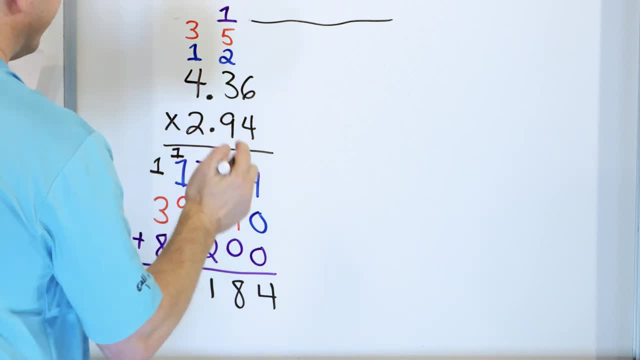 We have 2 digits after the decimal here. 2 from here That means 4.. So we have to put the decimal right here for 4 positions after in our final answer: 12.8184.. So we have again 4 digits. 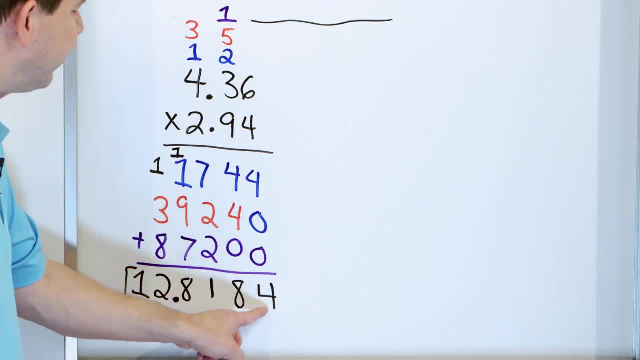 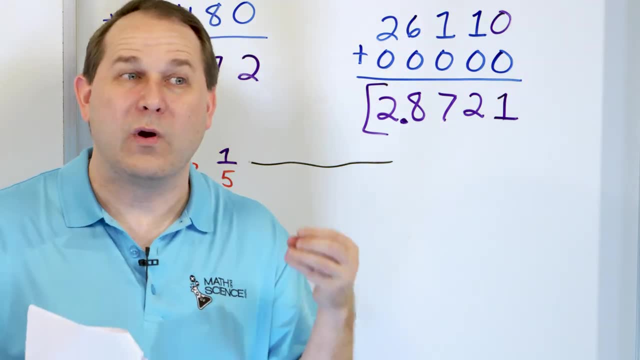 Tenths, hundredths, thousandths, ten thousandths. So again, this 4 means very, very little because it's so far toward the end. Every number there is only worth a ten thousandth, That's 1 out of 10,000 of something. 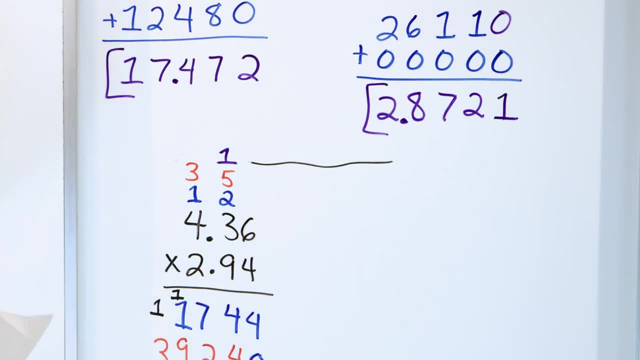 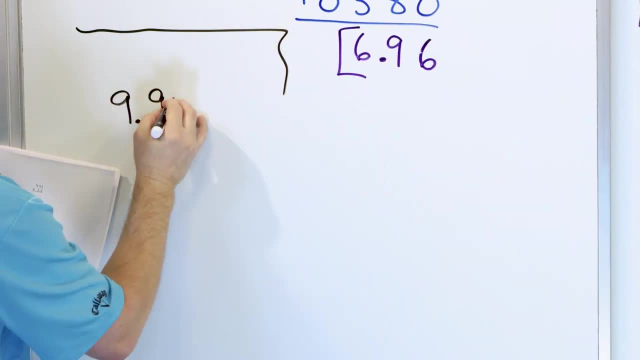 It's not worth very much, And so that's the final answer. All right, We only have one last problem, and we're going to work it over here. Let's take a look at 9.91 and we'll multiply it by 1.2, 1.2.. 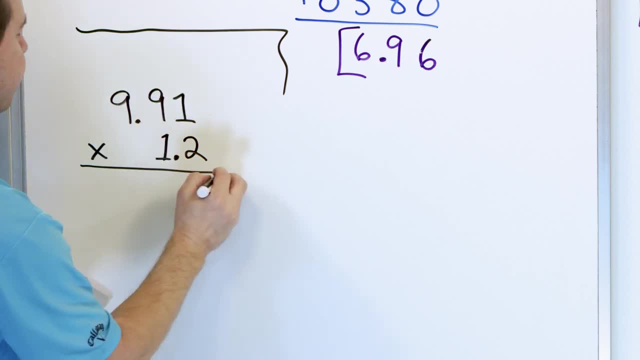 Notice: the columns line up with the digits. The decimals do not line up. All right, So first multiply by 2. 2 times 1 is what? 2. 2 times 9 is 18.. So we carry a 1.. 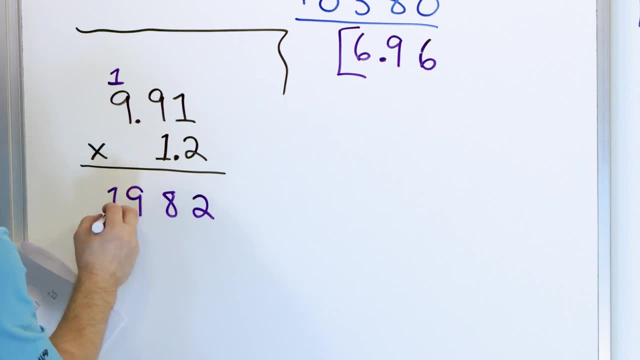 2 times this, 9 is 18.. One more is 19.. So there's your 19.. Multiply by 1.. We have to drop a 0.. 1 times 1 is 1.. 1 times 9 is 9..